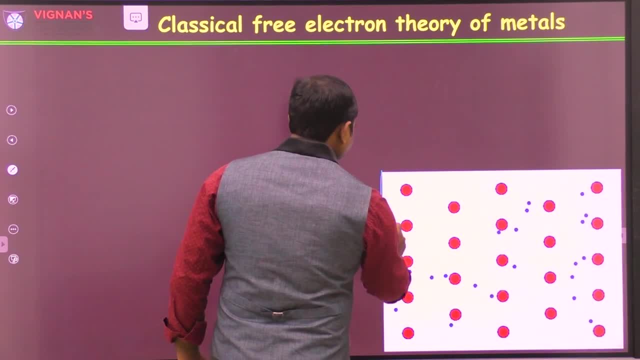 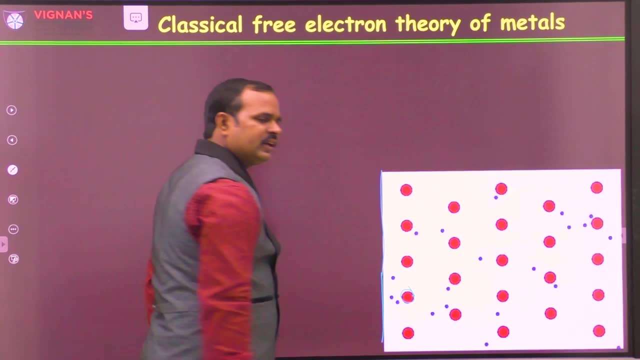 You can see here, this is a metal. In this metal these are all the atoms and these moving particles are the free electrons which are moving freely As per the assumptions of the classical free electron theory, that is a Drude and Lorentz. these are the atoms in the metal and then these are all free electrons. 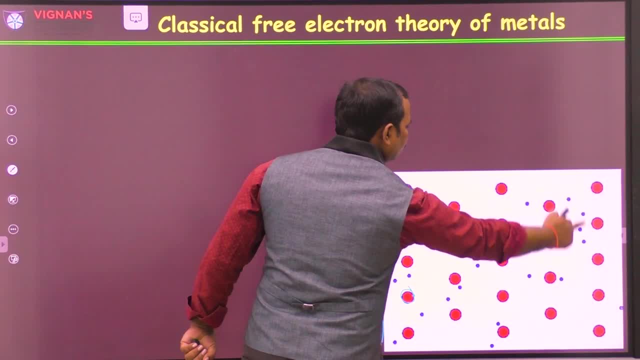 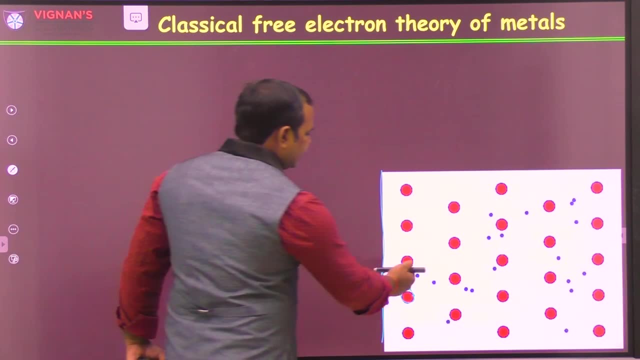 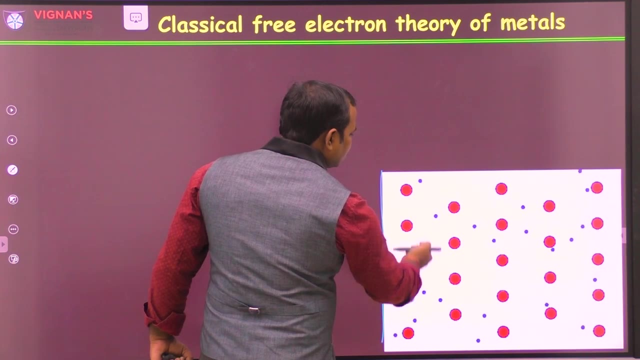 And all these free electrons are randomly moving throughout the volume of the metal under the absence of the external electric field. Now, these electrons, during their motion they can collide the atoms or the ions Also, the electrons can also collide with the other electrons. 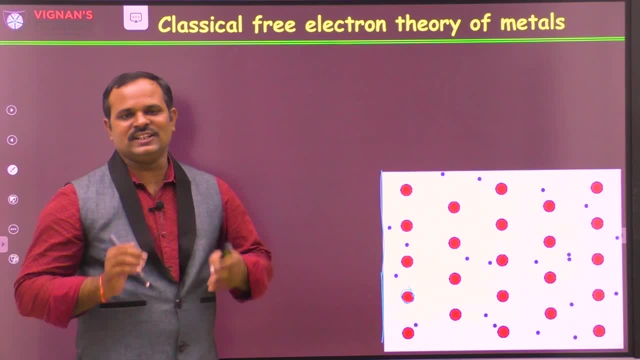 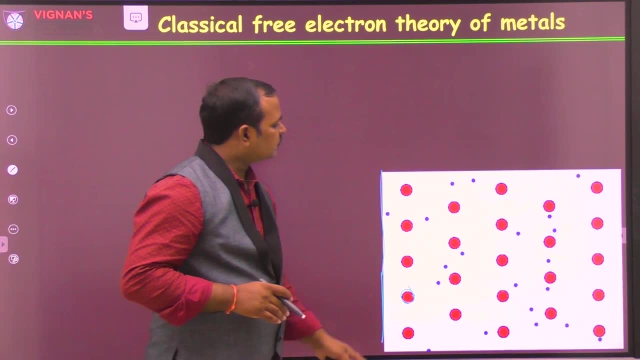 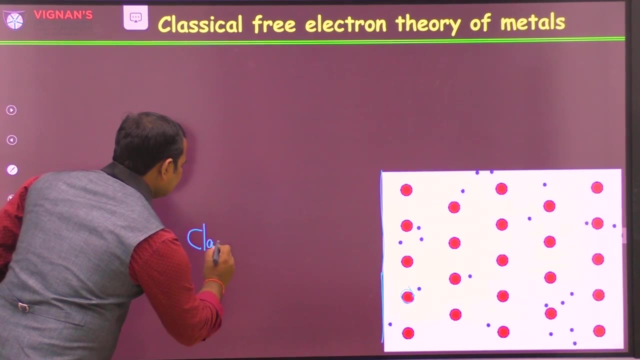 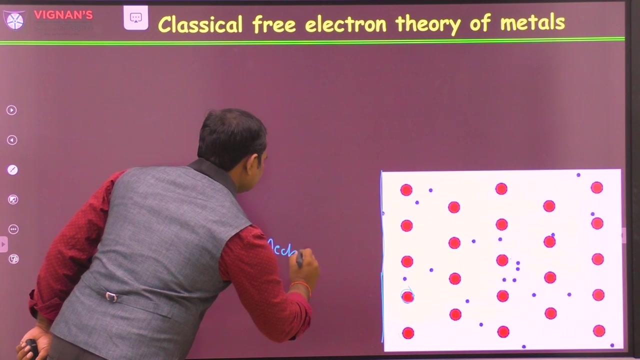 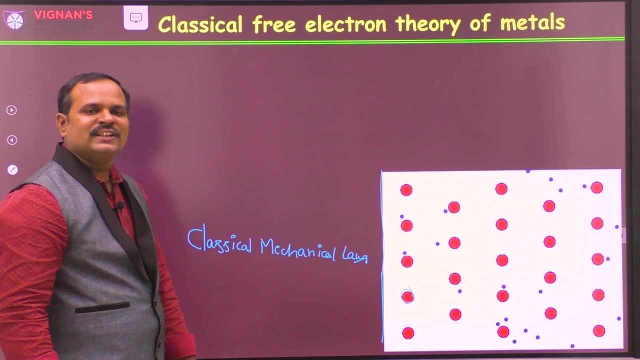 And these all collisions are purely elastic in nature. that means there is no loss in energy, and then the energy is conjured completely, and also momentum, And also now these electrons, follows classical, classical mechanics, Classical mechanical laws, Those are classical kinetic theory of gases, because these electrons are moving freely, like a gas molecules in a container. 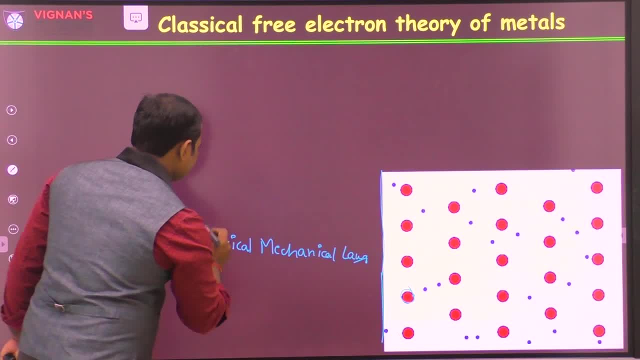 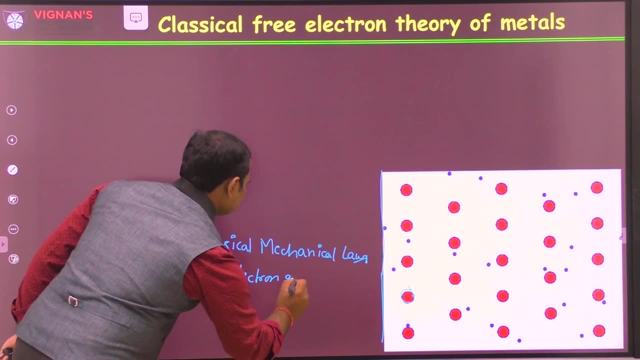 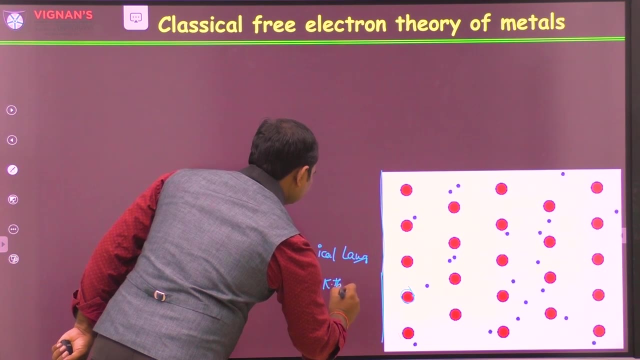 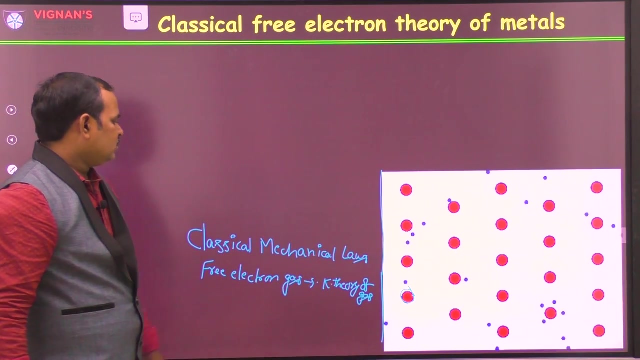 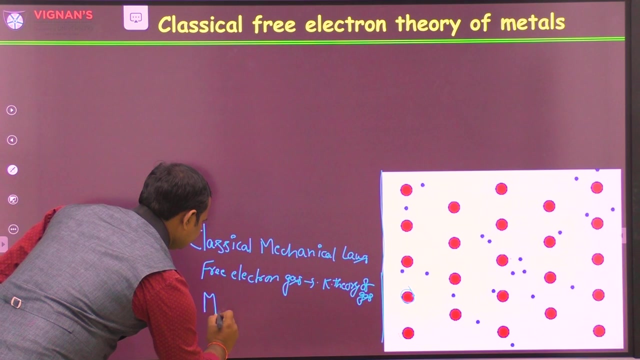 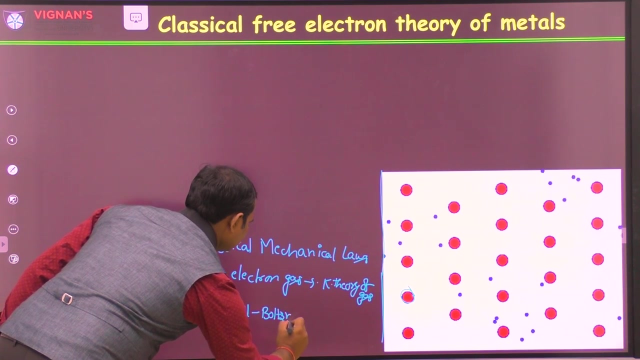 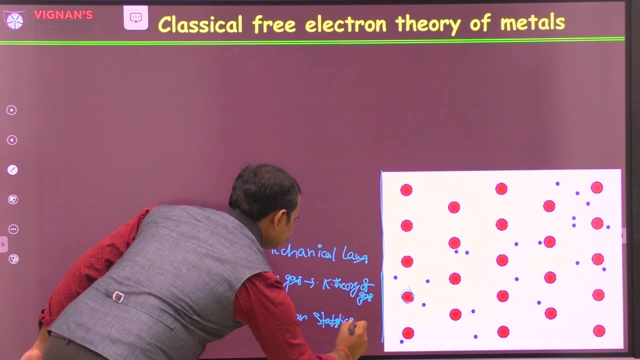 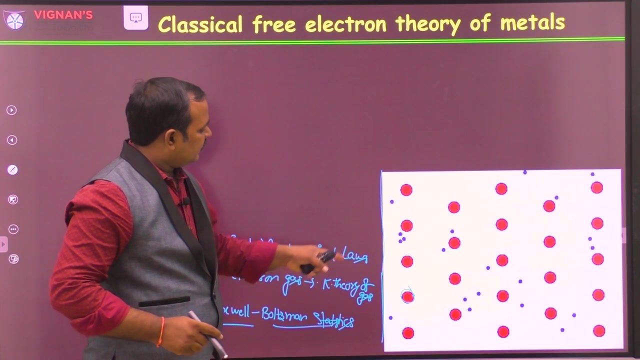 So he said that all these free electrons are called free electron gas and follows kinetic theory of gases, molecules and also all these electrons follows Maxwell-Boltzmann statistics. This is a classical statistics. Now, these are the assumptions that the Drude and 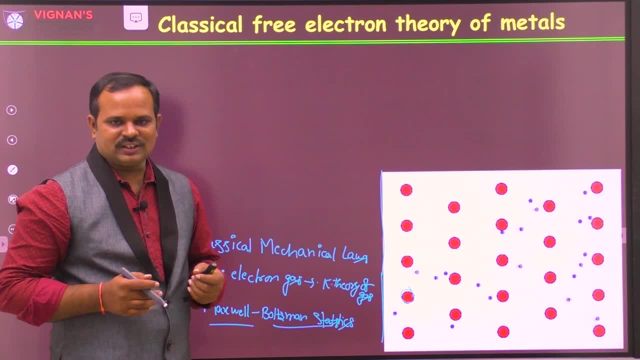 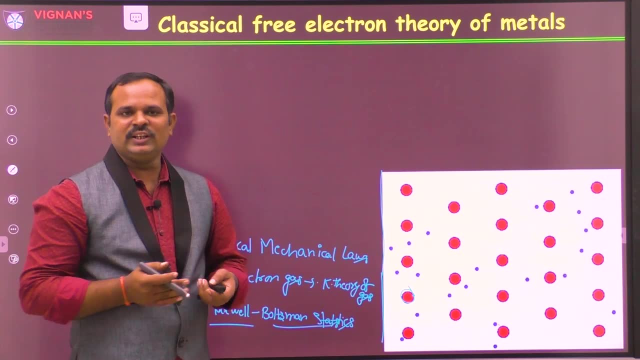 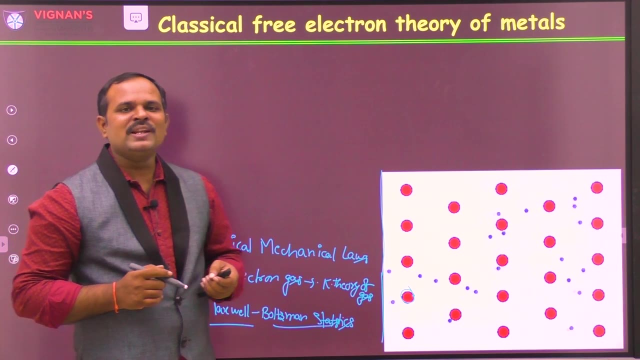 Lorenz assumed and then calculated the electrical conductivity and also based on these assumptions they could explain successfully the electrical and thermal conductivities of the metals, also some optical properties of the metals, malleability and ductility of the metals and so on. they also tried to to 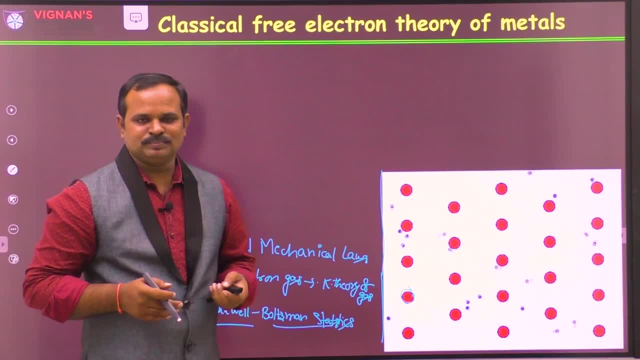 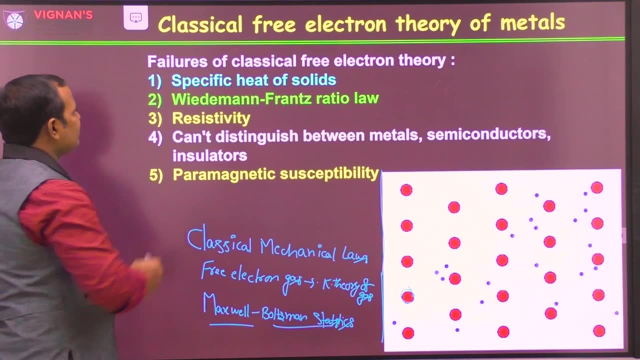 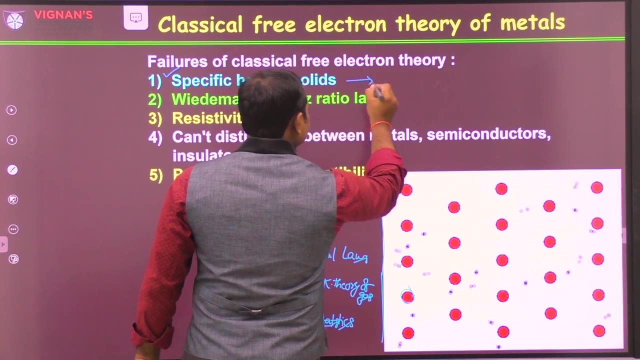 explain the Weidmann-Frange ratio law up to some extent. however, they have a lot of failures. you, you, You can see here the failures of the classical free electron theory, the specific heat of solids. The specific heat of solids is: according to this theory, the specific heat of solids is 4.5 R. 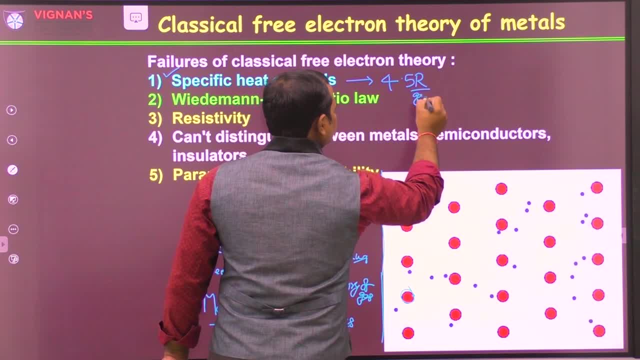 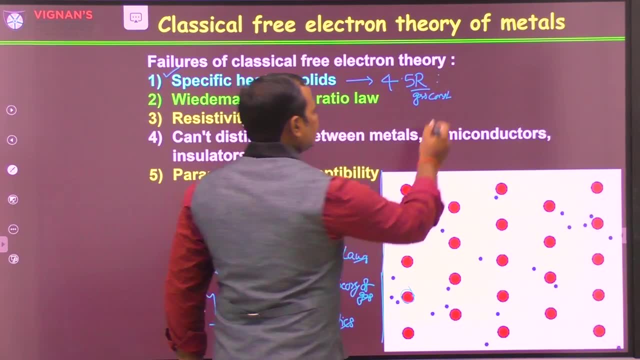 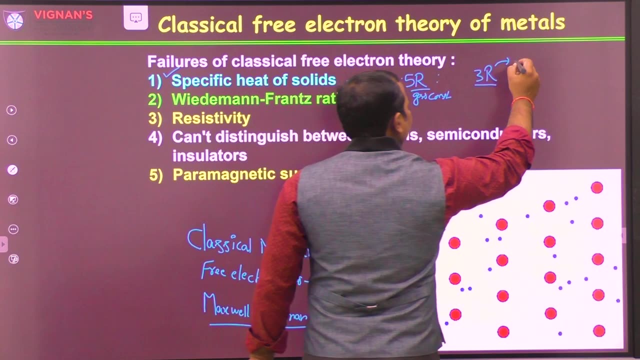 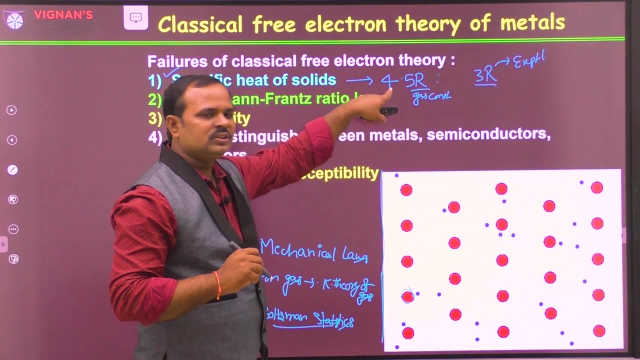 where R is the universal gas constant, But in general the specific heat of the solid is at and above room temperature, 3 R. This is the experimental. However, according to this theory, we got 4.5 into R. Now this could not be explained by using classical free electron theory. 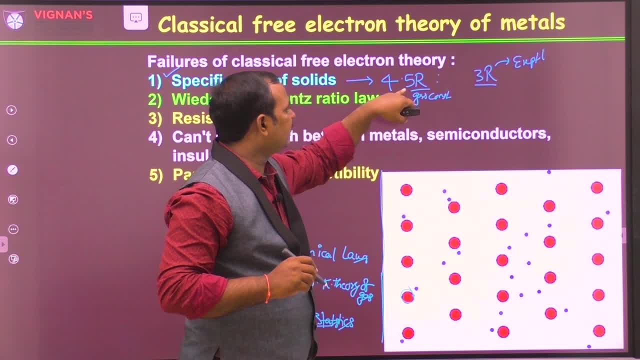 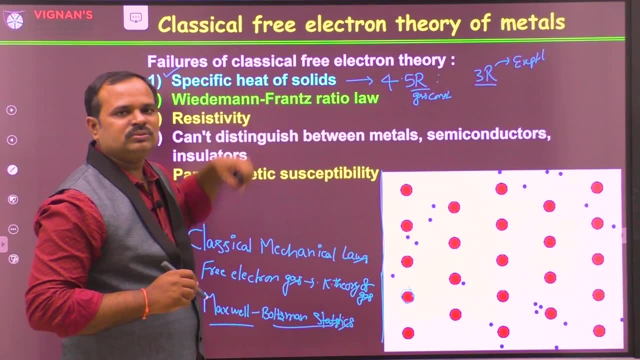 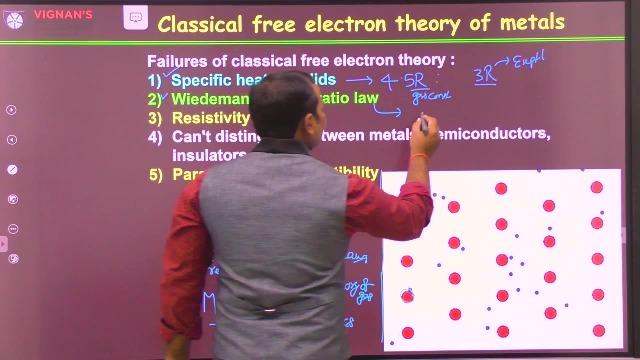 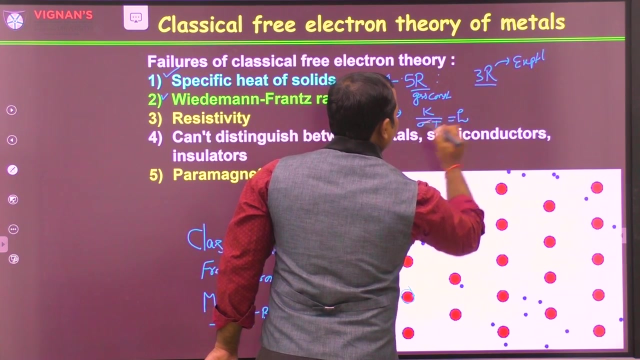 Why the discrepancy between the experimental value and the theoretical value calculated by using Drude and Lawrence, could not be explained by using classical free electron theory And then Weidmann-Franzi ratio law. This is the ratio between thermal conductivity to electrical conductivity at a particular temperature, is called Weidmann-Franzi ratio law. 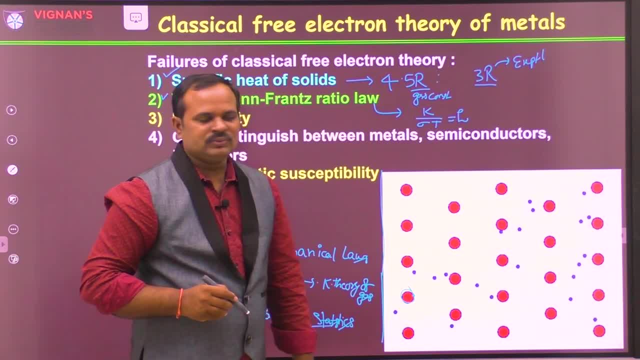 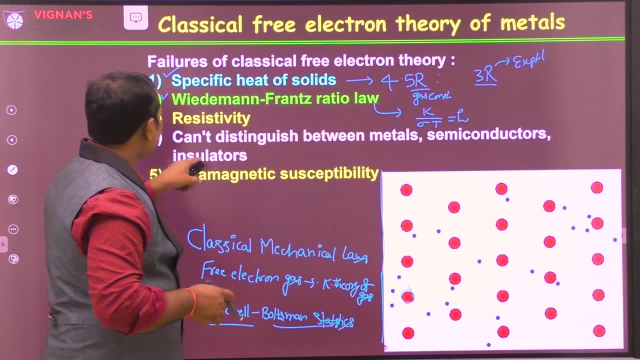 That is k, by sigma t. That is a Lorentz number. However, up to some extent this was explained, but it was not explained fully. Also, the resistivity of metals. The resistivity of the metals is explained, However. 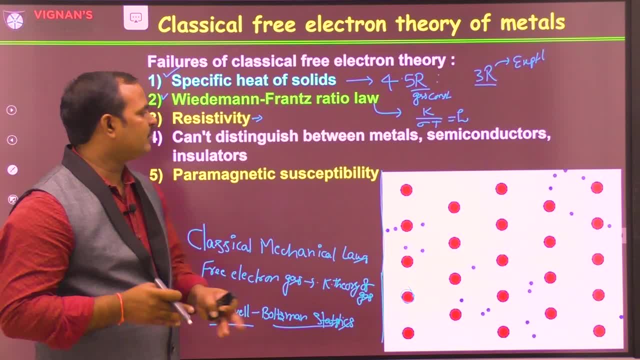 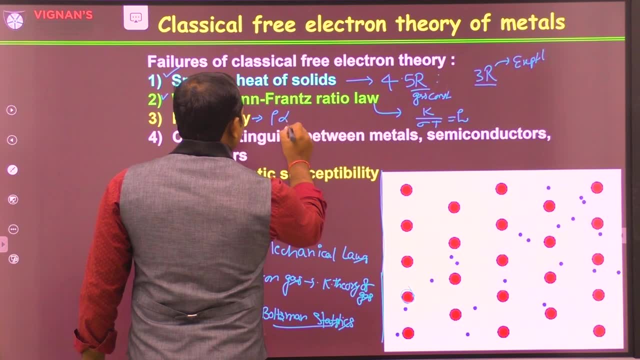 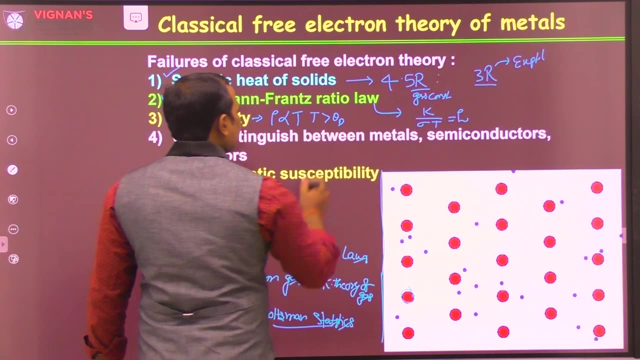 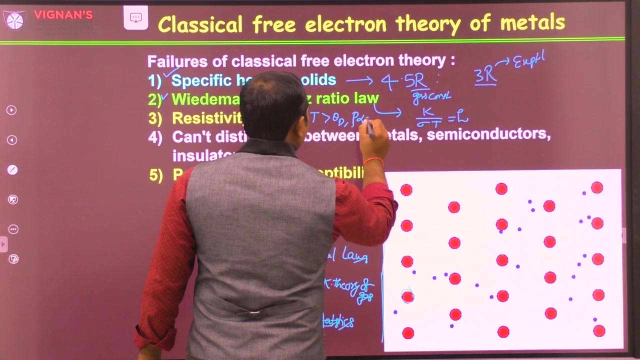 the temperature dependence of the resistivity is not explained by using classical free electron theory. In general, the resistivity is directly proportional to temperature when T is greater than theta d, And also the resistivity in the low temperature region Rho is directly proportional to T power 5.. 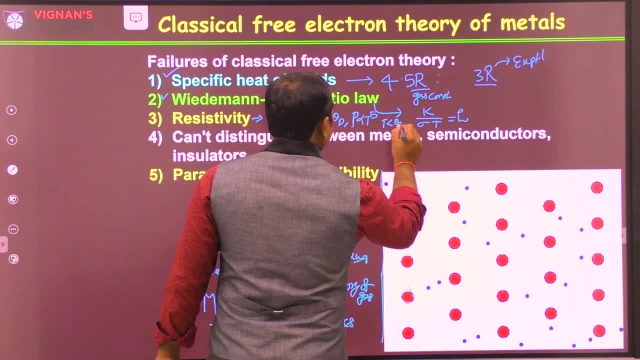 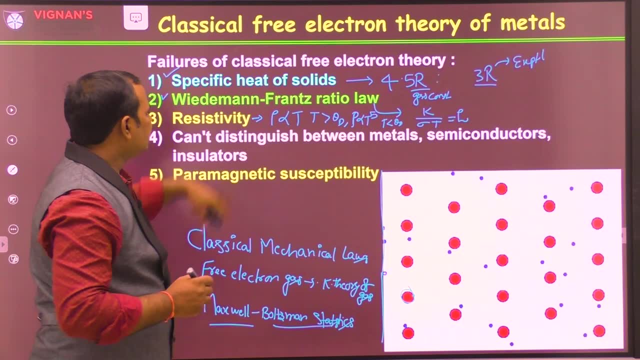 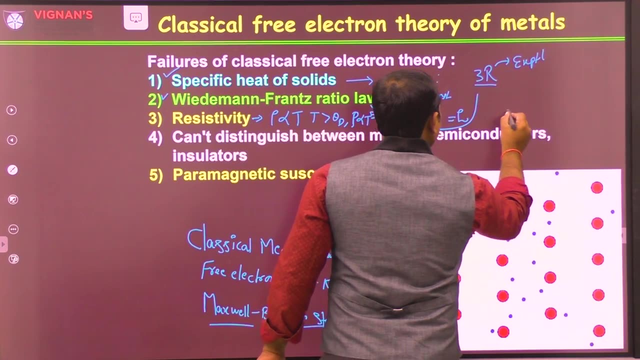 When T is less than theta d. This is how, in general, the resistivity, experimentally, we can determine. However, these theories. this theory was shown that resistivity is directly proportional to square root of T. That means T power 1 by 2.. 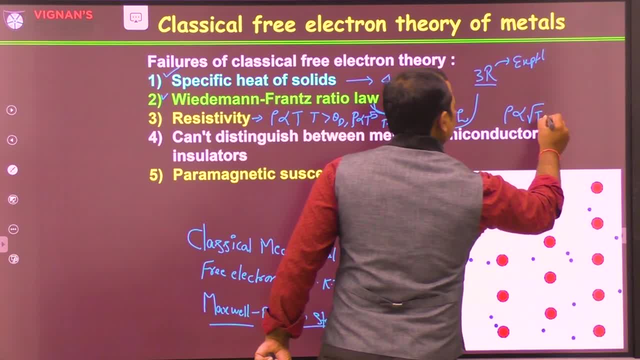 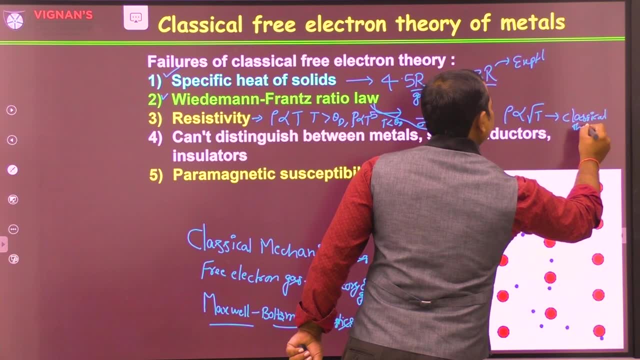 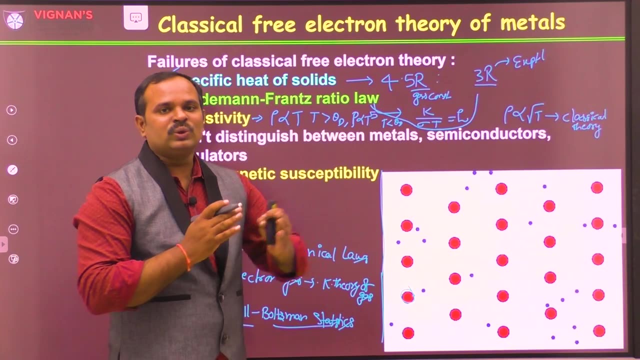 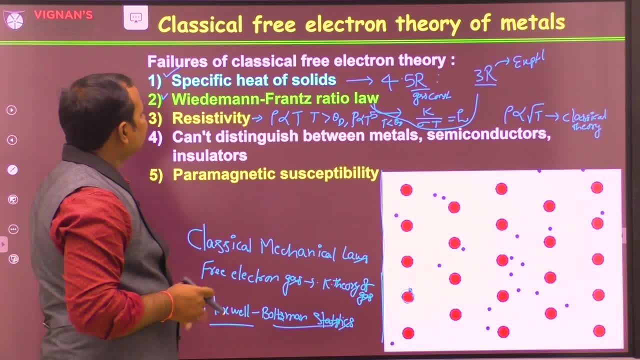 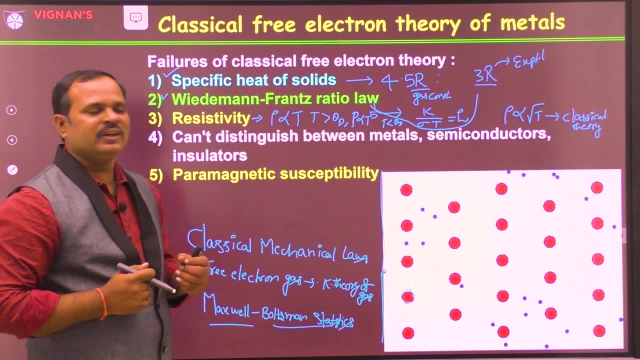 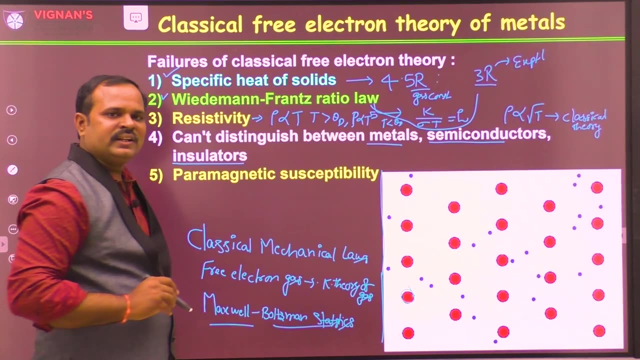 So this is also a failure. Another one is this theory is unable to. that means classical free electron theory is unable to distinguish between the materials like metals, semiconductors and insulators. Why some materials Or behaves like a metals, semiconductors and insulators. 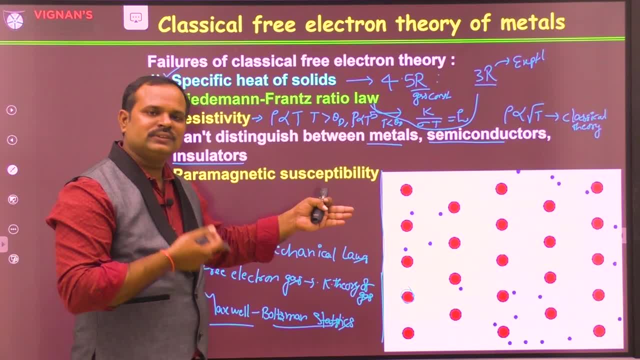 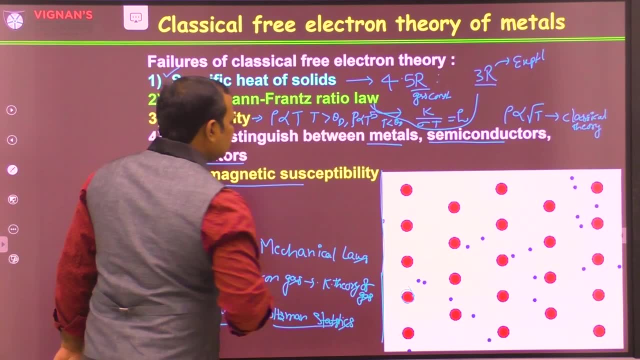 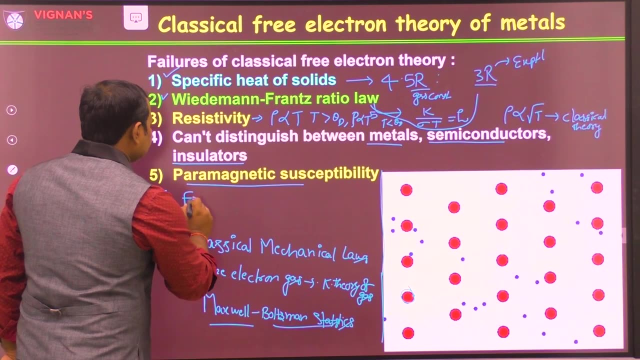 There is no way this Drude-Lorentz theory could distinguish between all these things. Also, the paramagnetic susceptibility is also not been explained by using this theory. Not only this, there are many things: ferromagnetism, ferromagnetism. 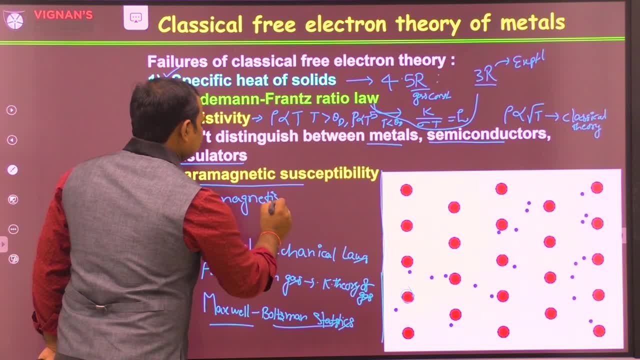 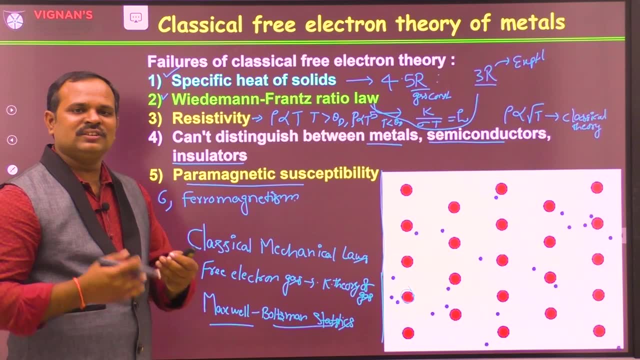 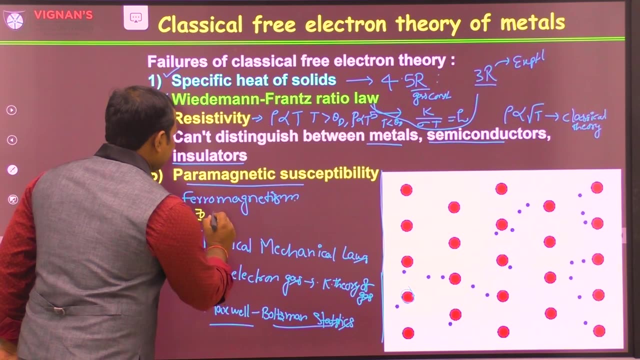 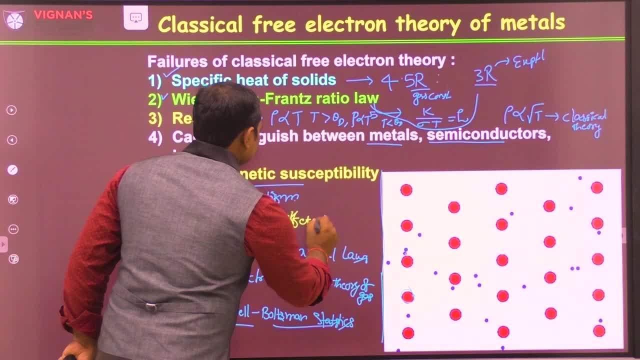 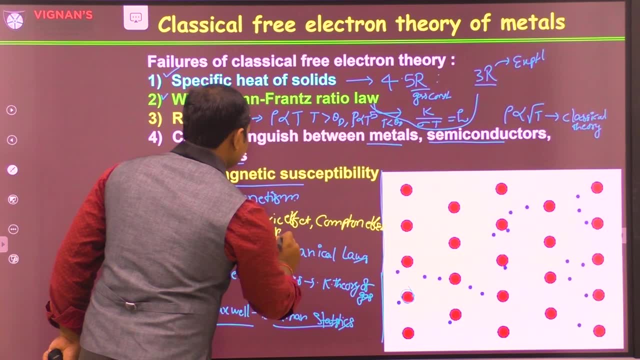 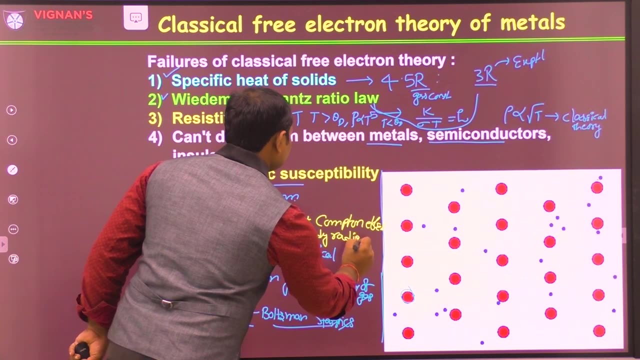 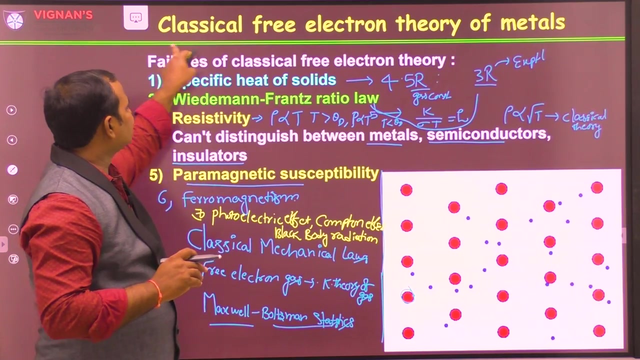 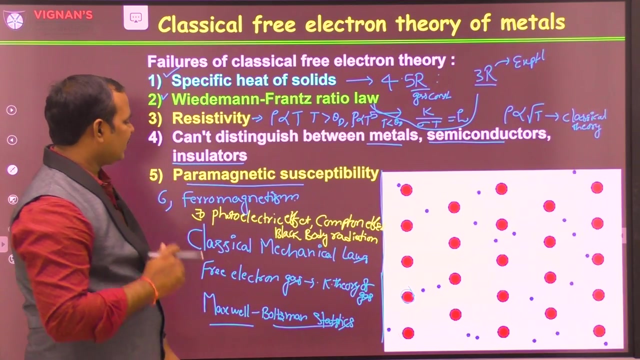 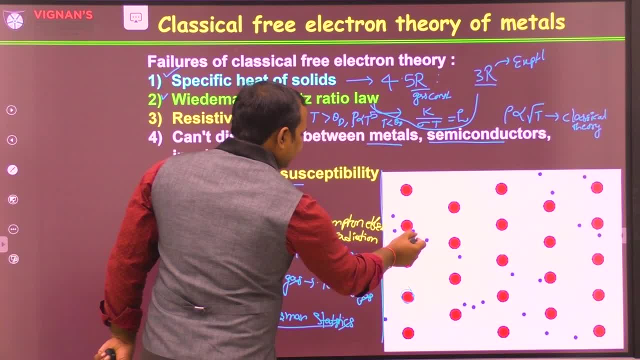 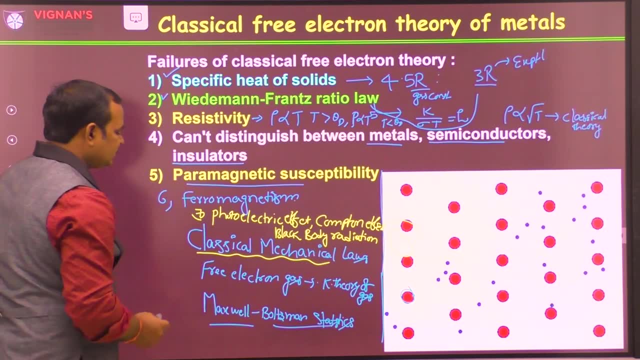 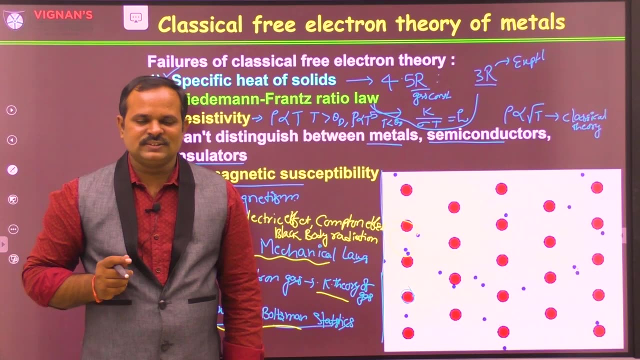 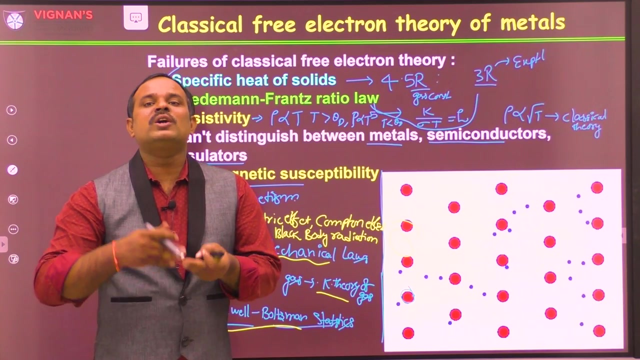 Drude and Lawrence assumed that all the electrons are. all these electrons are follows classical mechanics, Classical mechanics and follows kinetic theory of gases. and the distribution of electrons follows Boltzmann statistics. However, the electrons are quantum particles. We know already clearly electrons follows quantum mechanical laws. But Drude and 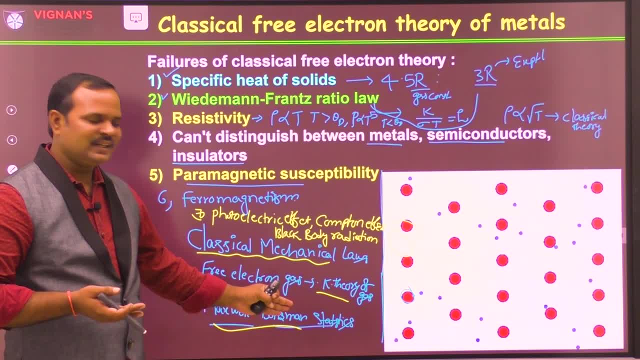 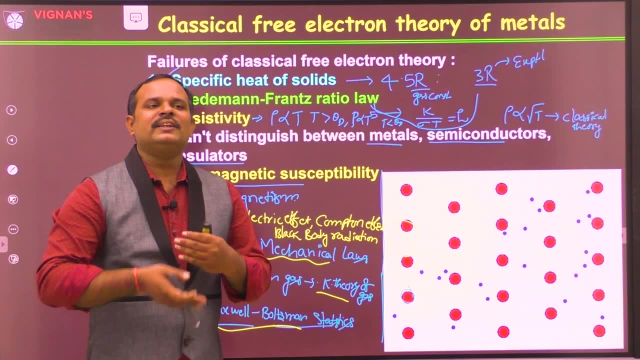 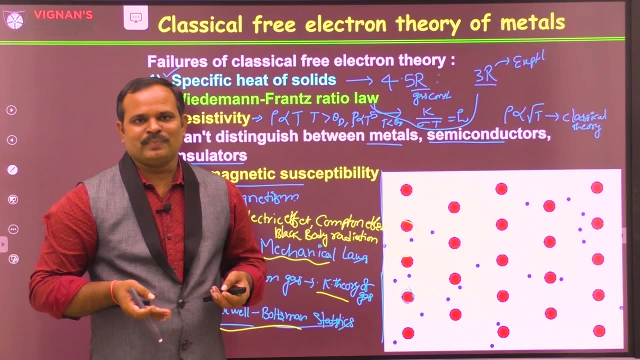 Lawrence assumed that the electrons follows classical mechanics. So they applied all these classical mechanical laws Onto the motion of electrons and then derived an expression for various physical quantities, So that there is a discrepancy Now in the quantum free electron theory, in the quantum 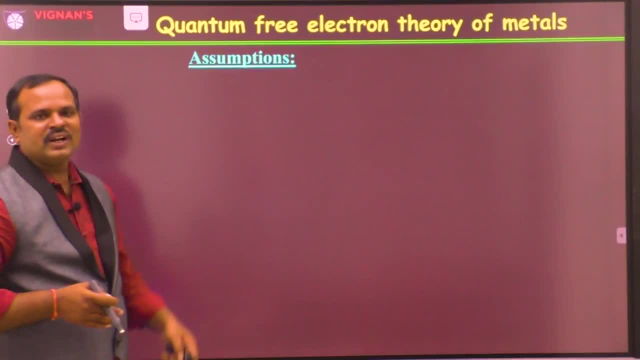 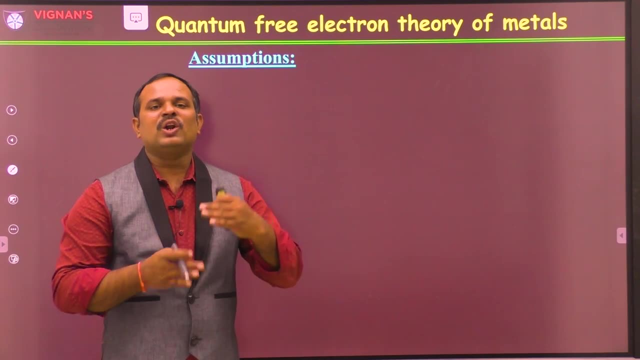 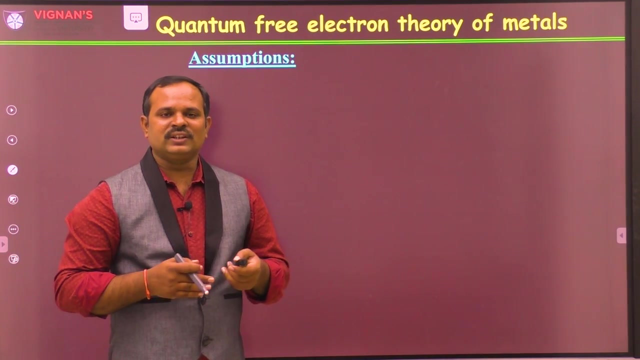 free electron theory. Sommerfield was introduced to quantum free electron theory. In this quantum free electron theory, Sommerfield assumed that all these electrons follows quantum mechanical laws. Let us see the assumptions of quantum free electron theory, which was done by Sommerfield. Let us see the assumptions. 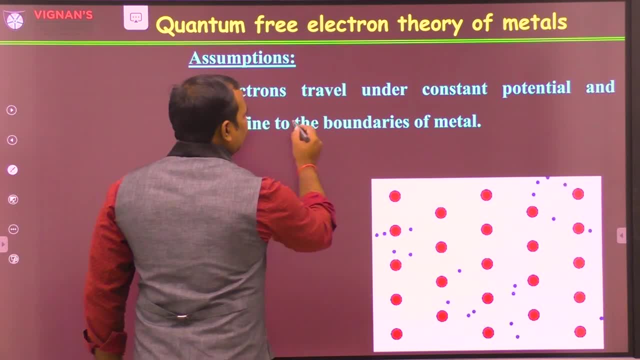 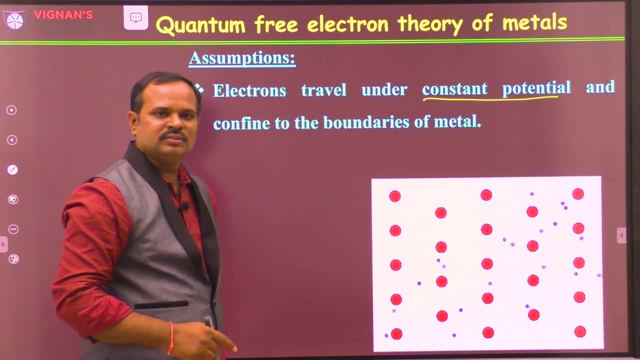 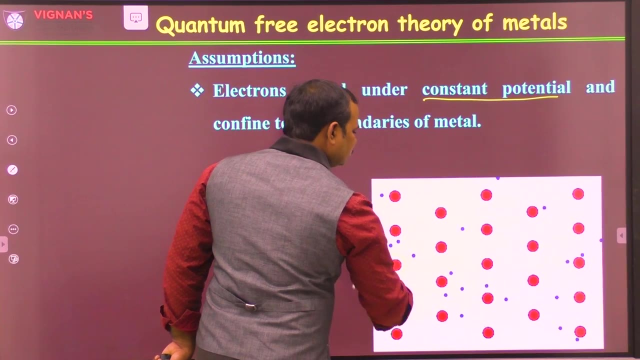 The first assumption is: the electrons travels under a constant potential in a metal- Here also consider, there is a metal. Every metal is composed of atoms. These all are atoms and all these electrons, free electrons, are called free electron. These electrons move throughout the volume of the metal under no external electricity. So in order to solve this, 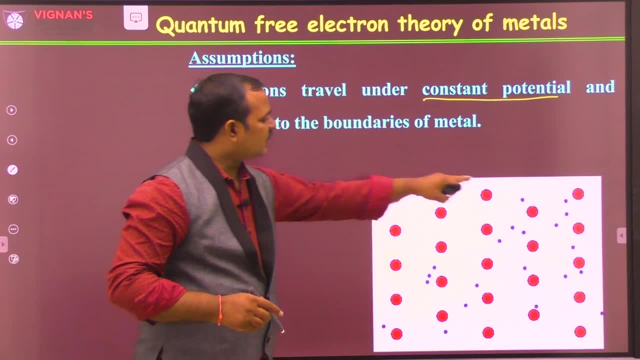 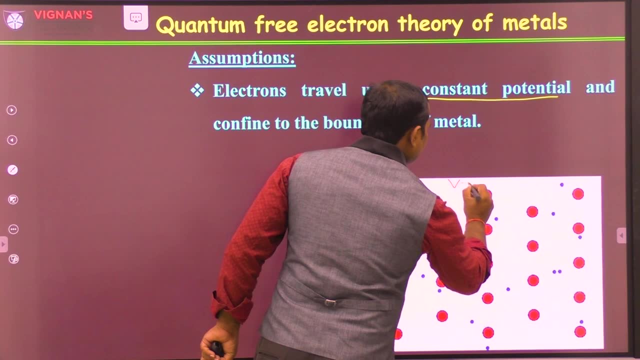 what is possible. orảng히 y hein. This is going to be the assumption of quantum free electron theory which was done by Sommerfield. Let us find out the assumption below. So the first assumption is the electrons field And these electrons moves under constant potential. V is constant. Maybe we can consider. 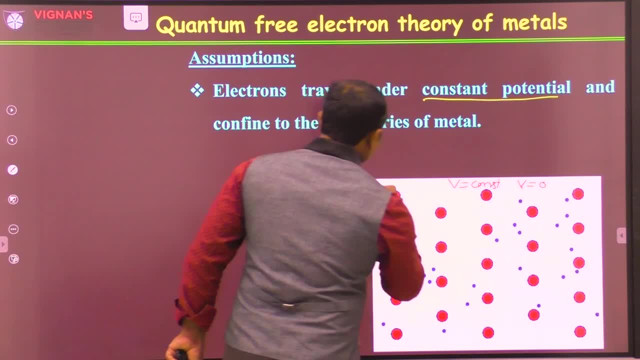 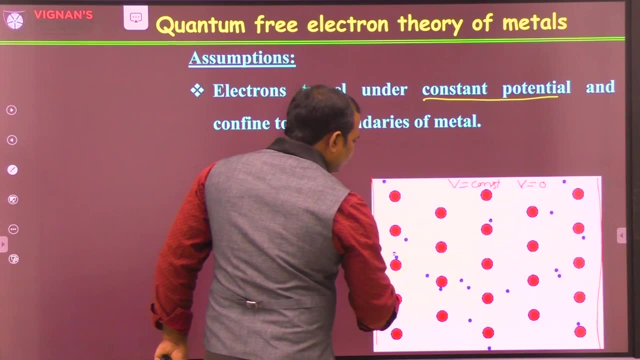 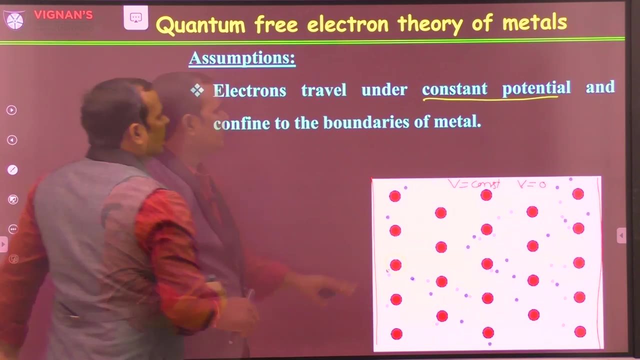 the constant is 0. That means from here. this is the edge of the metal, This is the edge of the metal. Within this boundary, the electrons can move freely from here to here under constant potential. That constant potential is 0. And confined to the boundaries of the metal, That's. 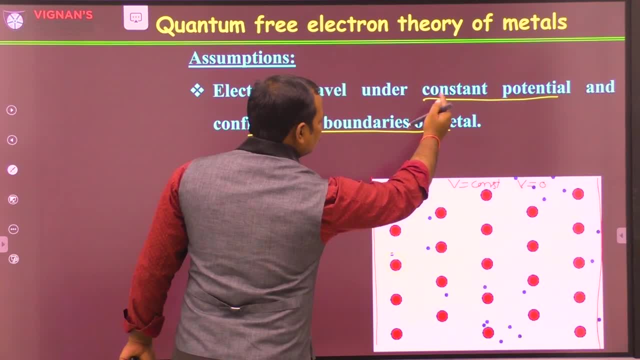 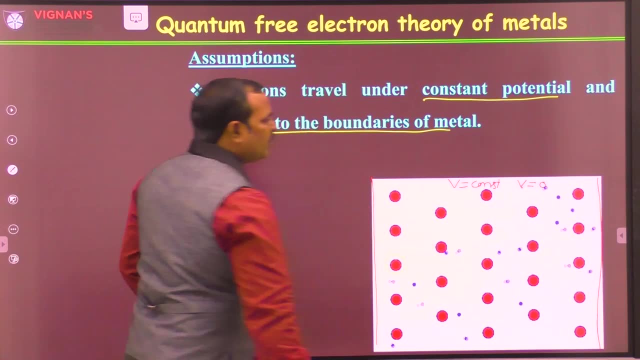 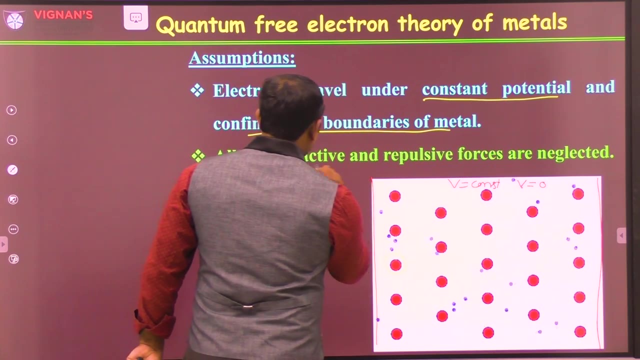 what. these electrons moves under constant potential- The constant potential term is more important- And then they can move freely throughout the boundaries of this metal. The second point is: all the attractive and repulsive forces are neglected. All the attractive and repulsive forces between the electrons and the positive ion cores are neglected. 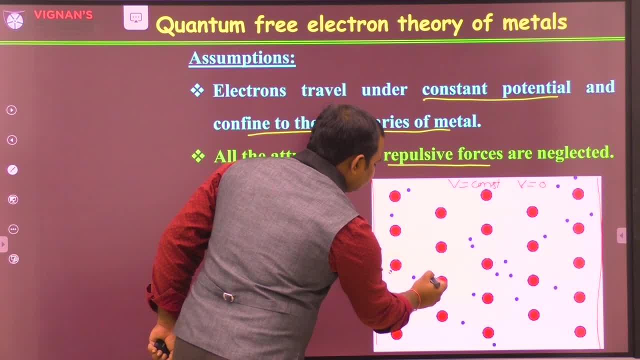 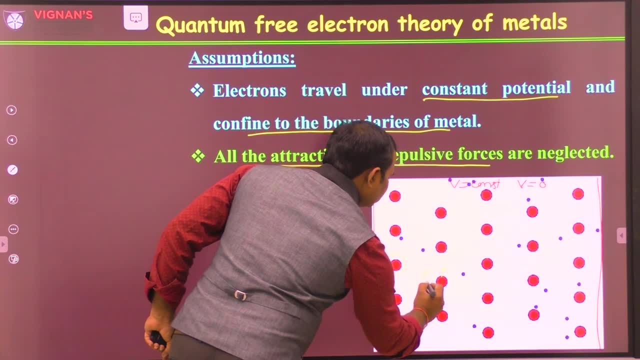 You can see here, when the electron is moving here, the electron has a negative charge And then ion core has a positive charge. Electron will have a negative charge, Ion core will have a positive charge. There is a force of attraction And also when the electron is colliding with. 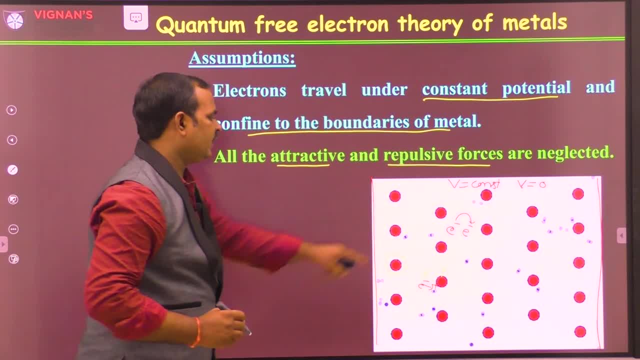 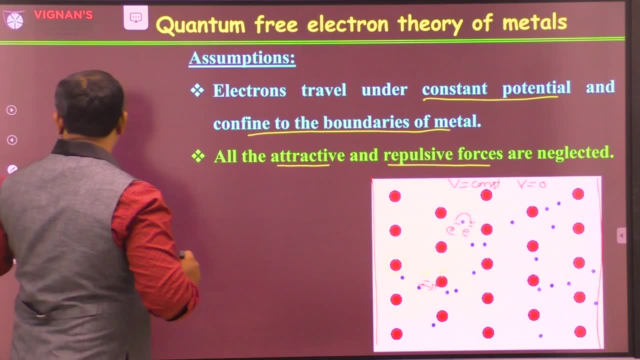 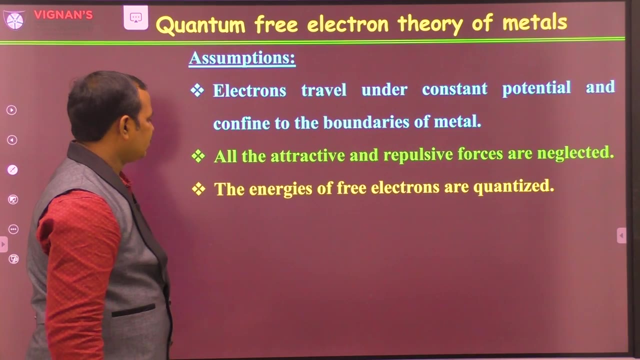 another electron. these two will have both negative charge. They will be repelling each other. All these kind of attractive forces and the repulsive forces inside this metal are neglected. So these are some of the assumptions you can see continuously. Now you can see here the third assumption. 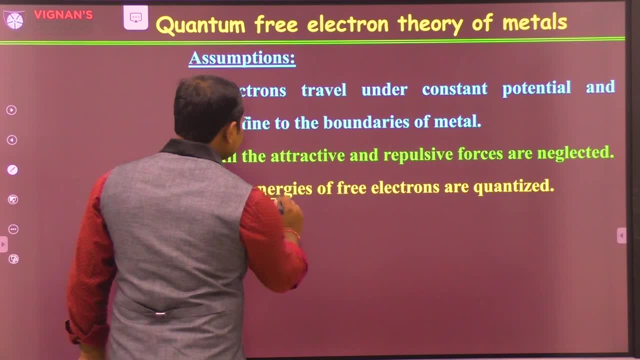 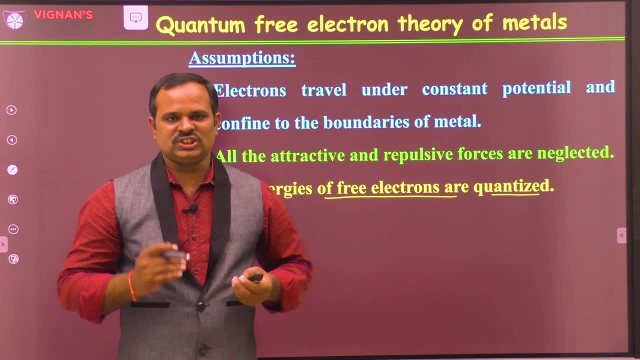 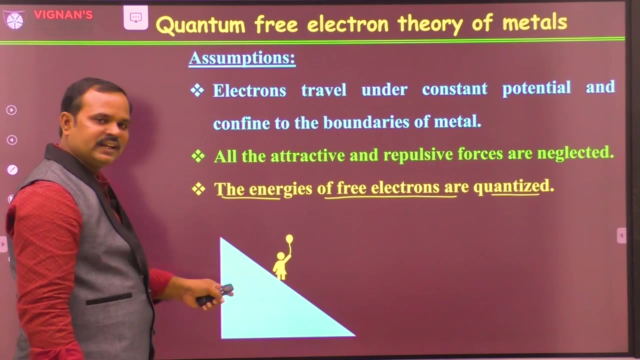 is, the energies of the free electrons are quantized. What is the meaning of quantization of energy? What is the meaning of quantization of energy? Let us see for this one in a simple example. You can see here: in this one, one person is climbing up In the same height. 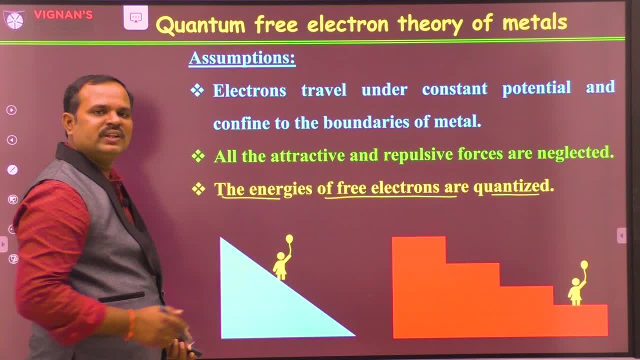 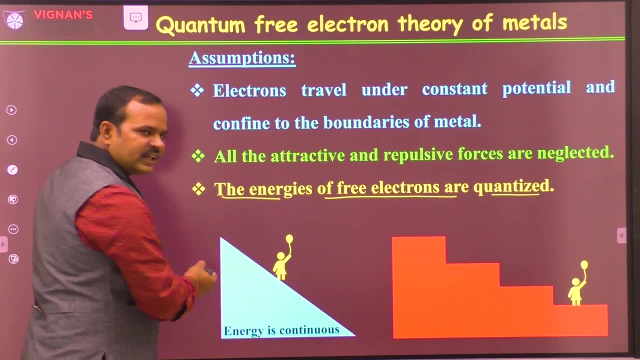 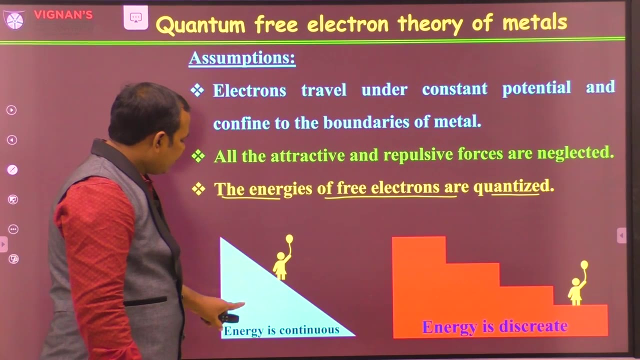 some other person is climbing In this way. What is the difference between these two? The main difference is: this is a continuous. You can see here, this is a continuous state And here you can see the discreteness. There is no continuous in this one, So we can say that the energy is continuous. 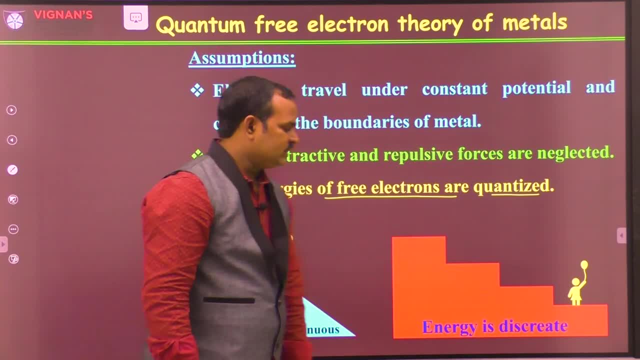 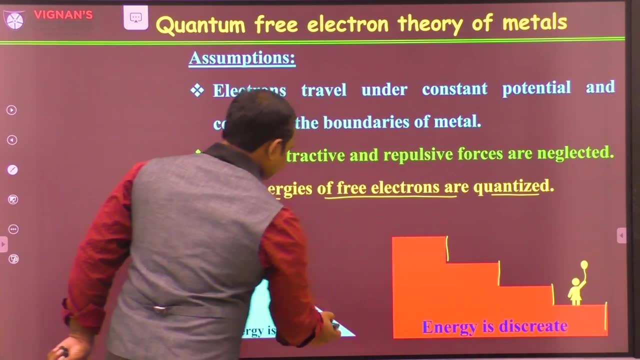 here And here, the energy is discrete. here, You can see, here, the possible energies are only from here and here. here, here is only, But here it is, you can see, there is a continuous, continuously energy needs to be spent. 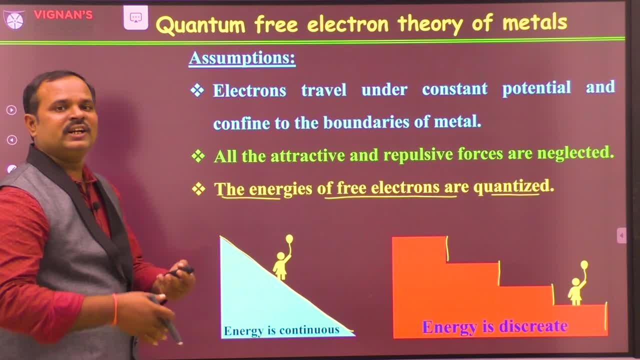 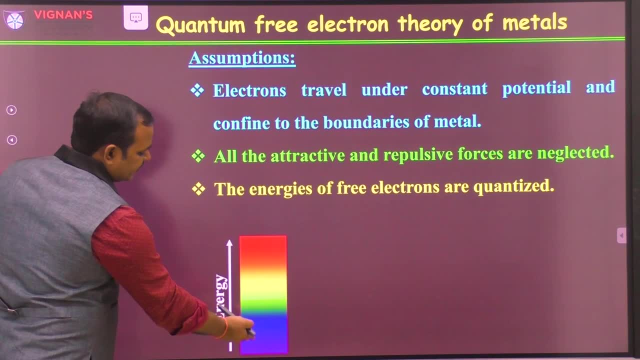 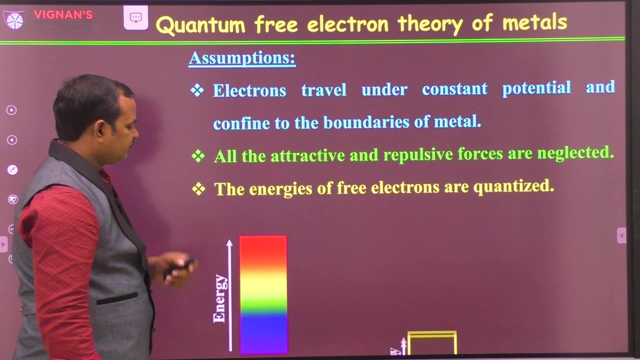 More clearly. we can see here in terms of energy and energy level diagram. This is an energy level diagram. The meaning of this one is: you can see here the color is continuously varying, So that means the energy is continuously varying. And here you can see according to: 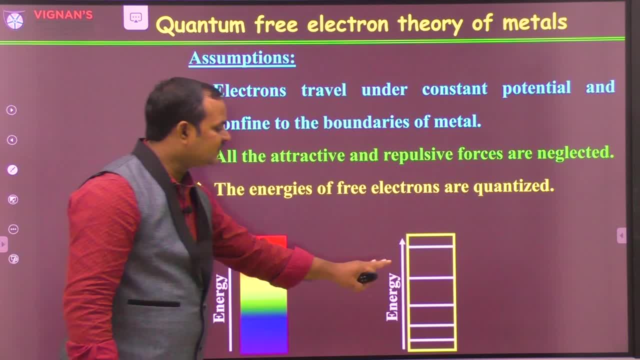 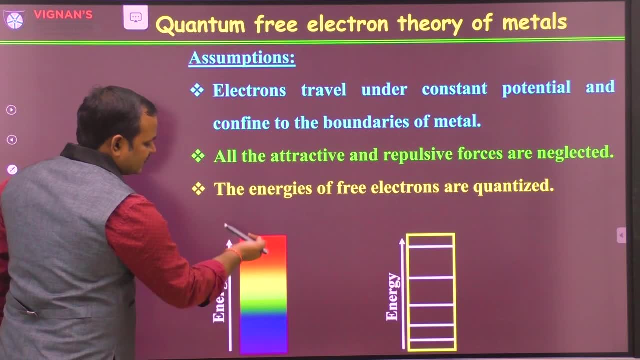 quantum mechanics. there is only the energy levels are existing in the system discreetly. You can see here. Here the energy levels are consisting in the mixed system. You can see here here-the levels are continuously existed. that means you can see, everything is the. 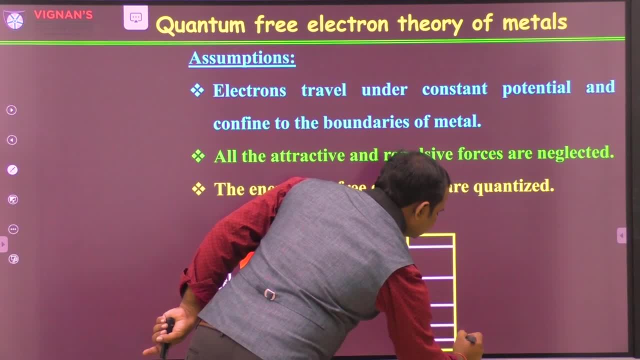 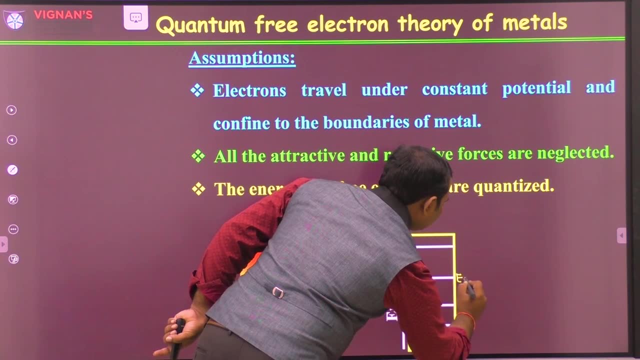 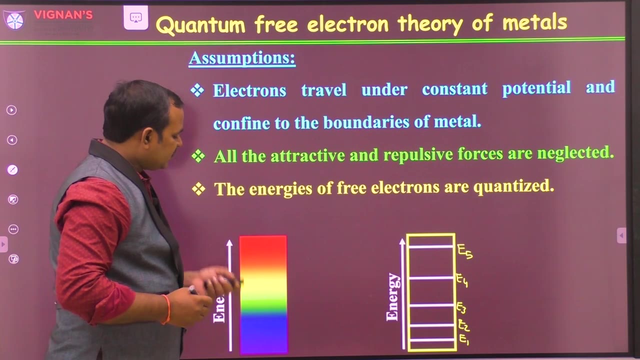 continuous energy, but here you can see, the energy is only existing. here this is a e1, this will be e2, this will be e3, this will be e4 and this will be e5, but here there is a continuous energy levels are there? so, because of this one, now we 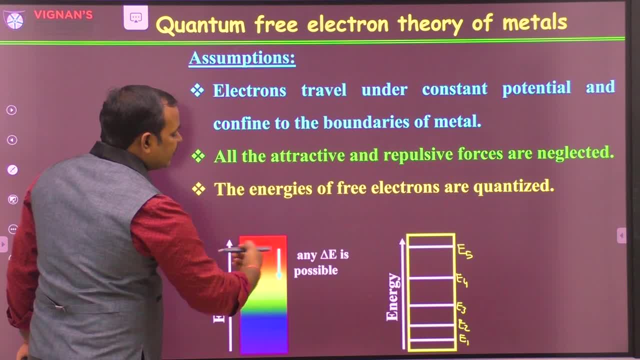 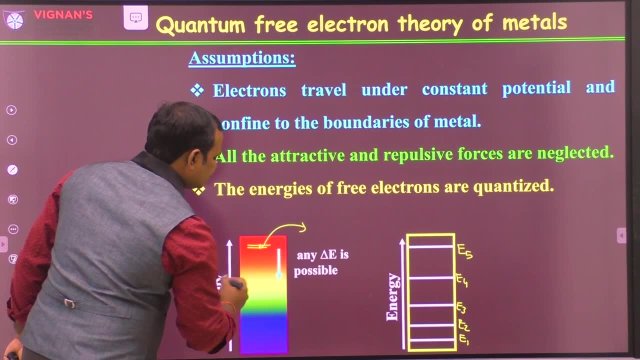 can get. any difference in energy is possible because of continuous energy. I can have the difference between these two energy levels also. the delta e. delta is changing energy. I can have difference in energy Silence. the difference between these two energy levels is also possible. another delta E, but whereas in this case there is only fixed certain delta, E is. 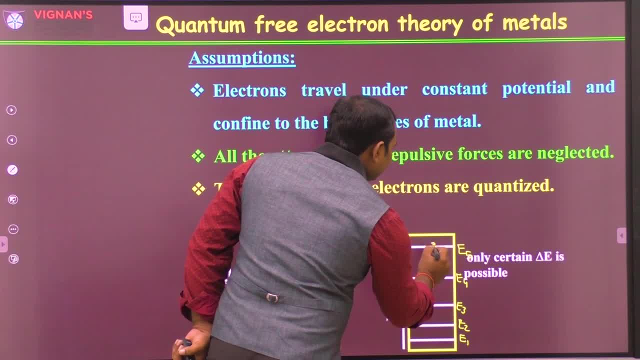 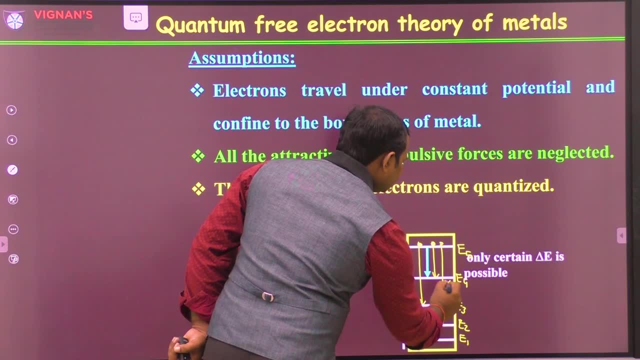 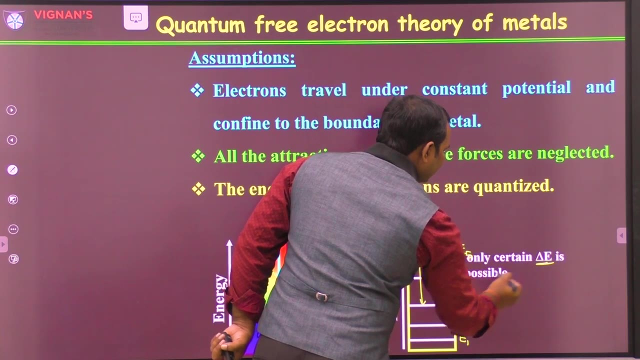 possible. that means either the electron or particle the jump from here to here, are here to here, but electron cannot jump from here to here because there is no energy here. So electron cannot jump, So only sometimes changing energy. that means delta E is possible in the quantum. mechanically This is because there is a discrete 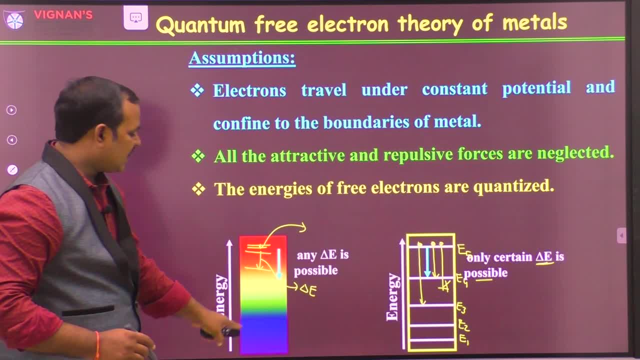 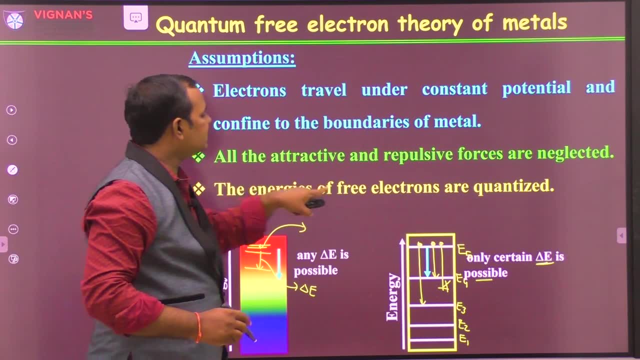 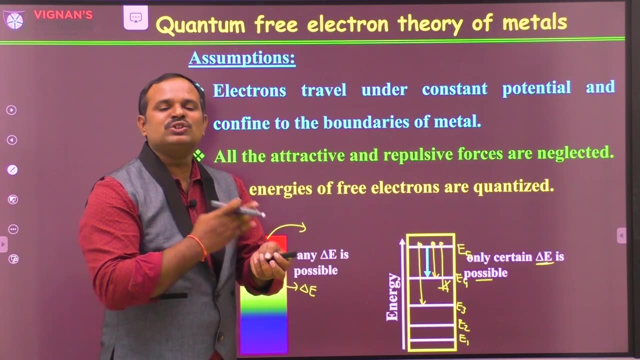 energy levels are existing. in the quantum mechanical system, In the classical mechanic system, continuous energy levels are existing. The meaning of the energies, the energies of electrons, are quantized means this is the one. Quantized means the discrete energy levels. and energy is quantized, That means the total energy of this system can be written in terms of small. 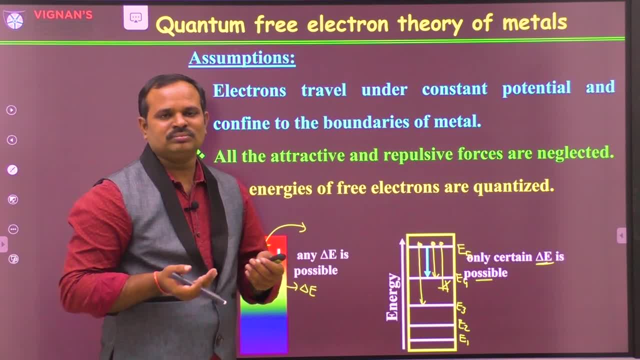 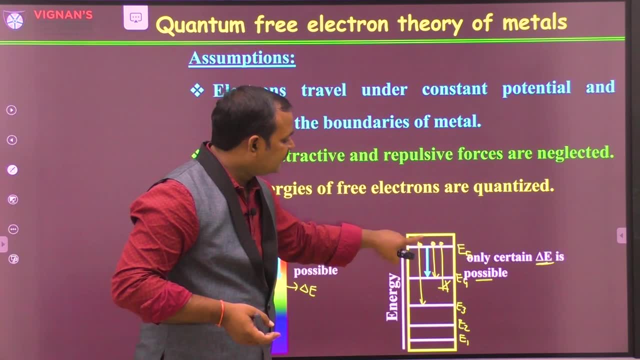 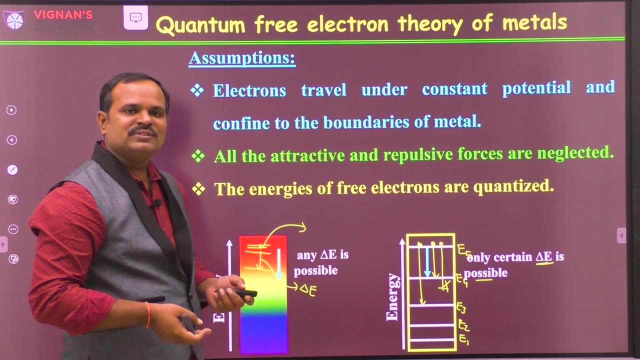 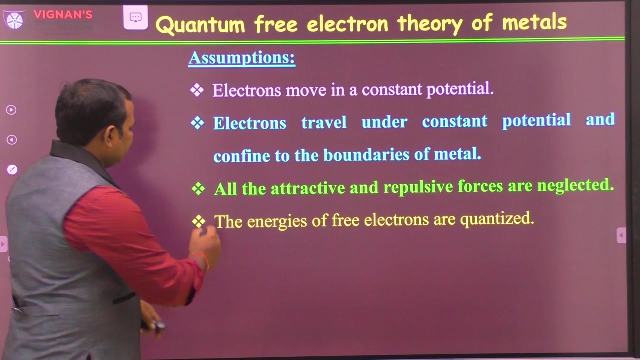 quantity, That small quantity is called quantum. So the total energy in this system is quantized And now because of this discrete energy levels we get a line spectrum, not continuous spectrum. We already have seen in the introduction of the quantum mechanics, these things. Now we have seen this one. Next, electrons. 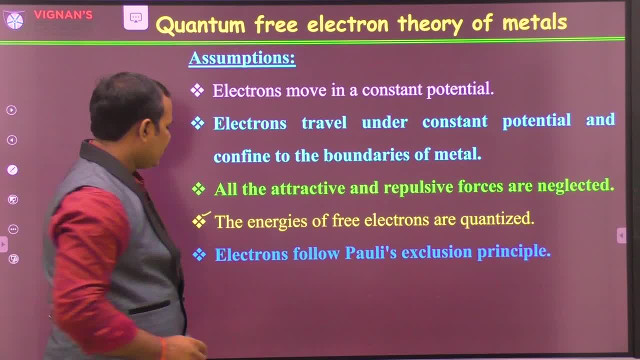 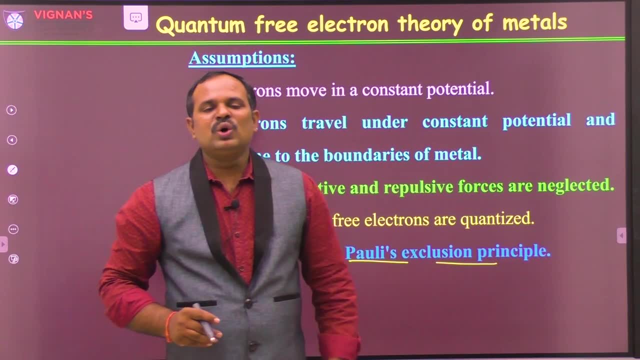 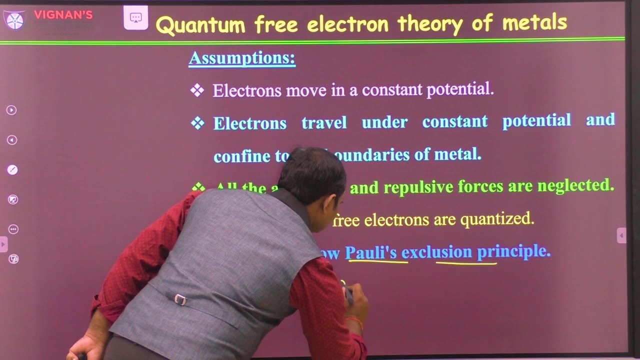 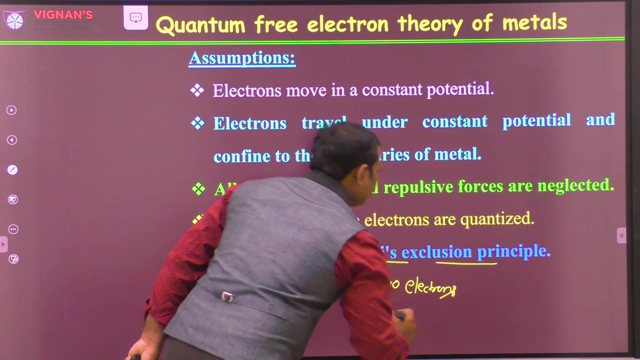 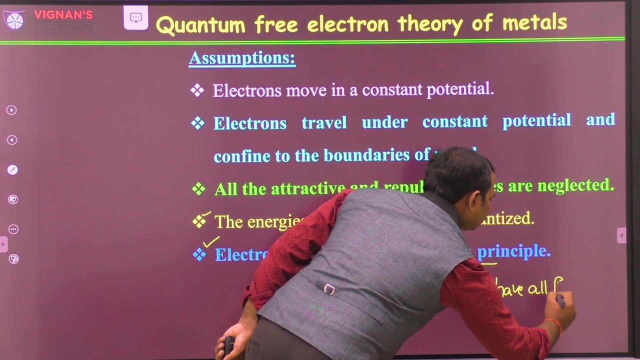 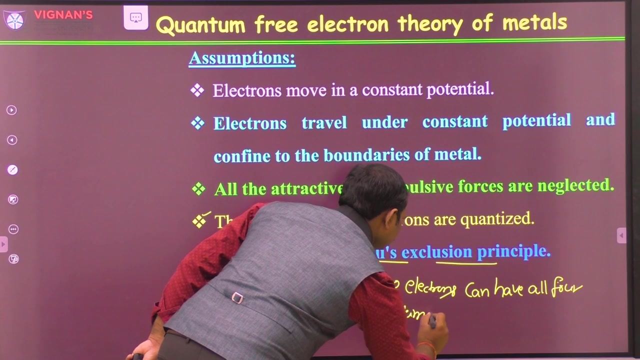 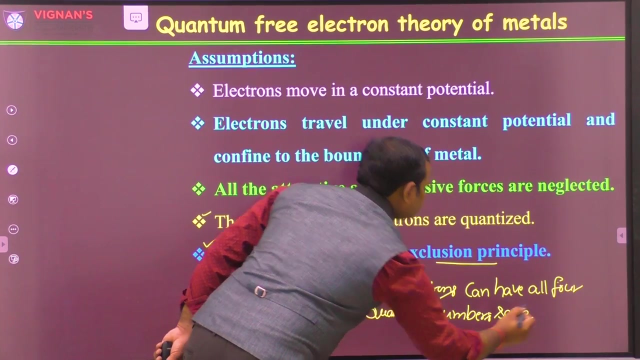 follows Pauli's exclusion principle. Electrons follows Pauli's exclusion principle. What is the Pauli's exclusion principle? No two electrons can have all four quantum numbers same. No two electrons can have all four quantum numbers same. This is the Pauli's exclusion principle. What is the meaning of this? 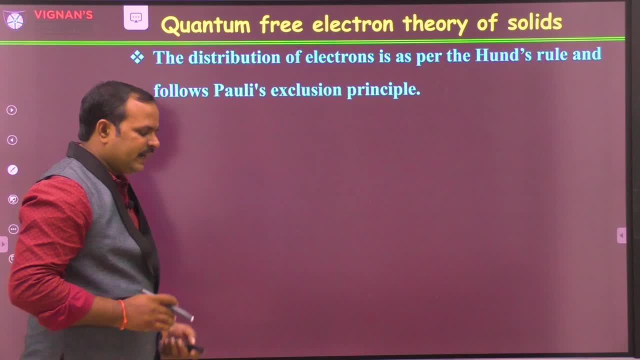 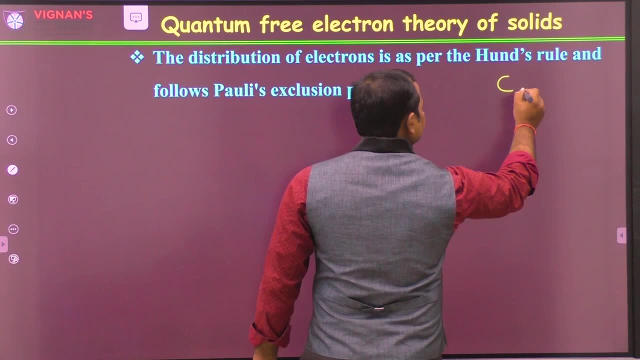 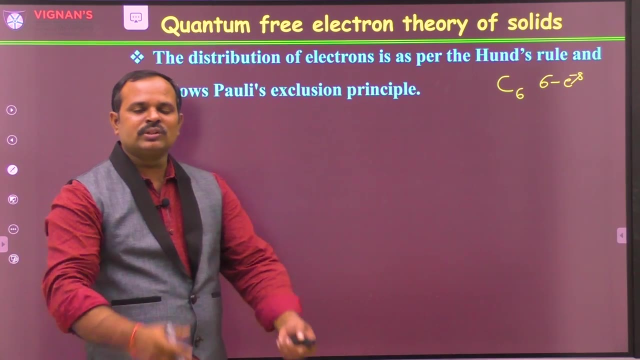 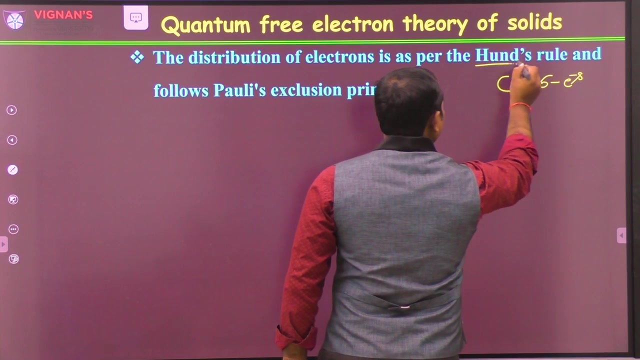 Let us see here, If you take a system- let us take, for example, carbon atom. Carbon atom contains six number of electrons- How these six number of electrons are distributed in different energy levels. This distribution of energy levels follows first Hund's rule and also Pauli's. 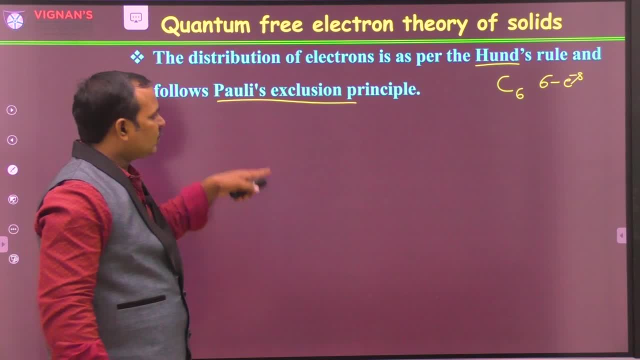 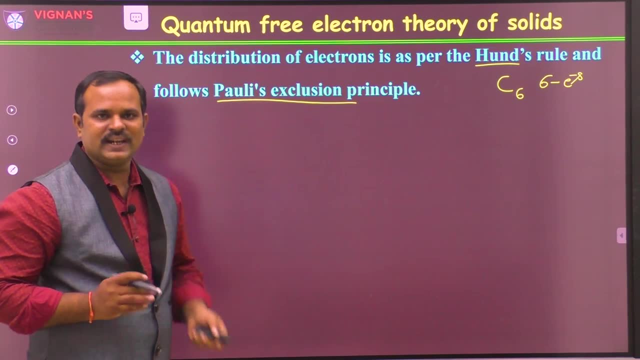 exclusion principle, Even in the quantum free books. it will be very simple: There isbst 들어 Gundười thicker. 어떻게 æ theory? the distribution of electrons or particles follows these rules. Let us see what is the. 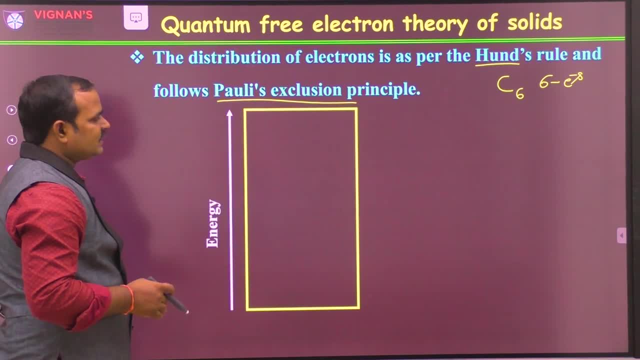 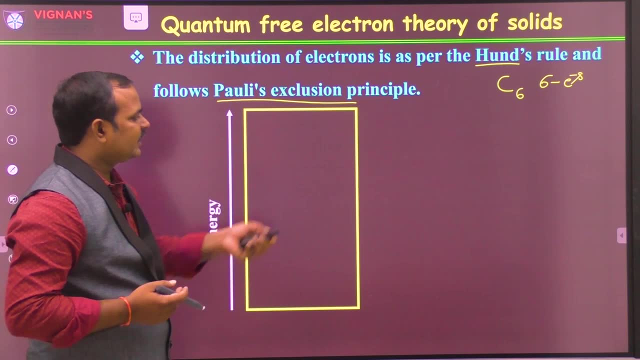 meaning of this You can see here. this is a. let us discuss first the classical mechanically, how the distribution can happen. That means the Maxwell-Boltzmann statistics. Later we will see how quantum mechanically the distribution changes In the classical mechanics we know. 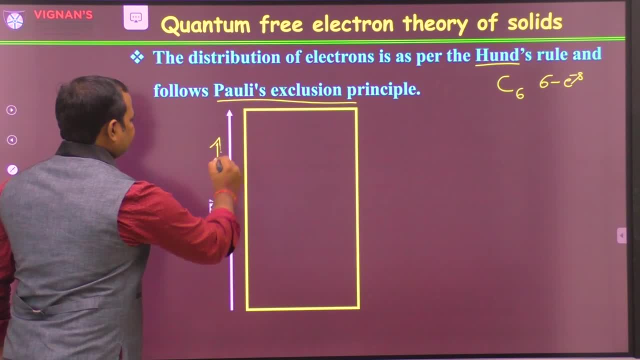 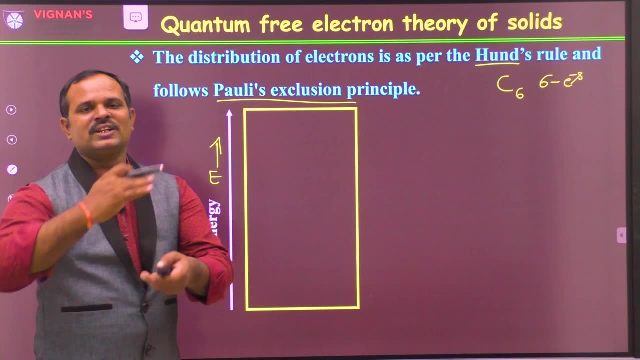 that these are the system. This is increasing energy. This is energy's increasing side. We know that the classical mechanics, every energy is possible. That means continuous energy levels are existing in the system. So this is the reason why there is a continuous 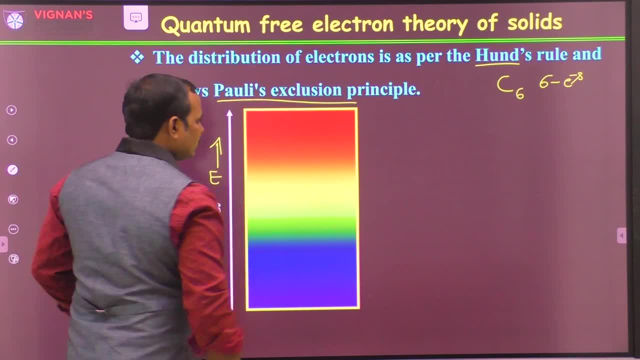 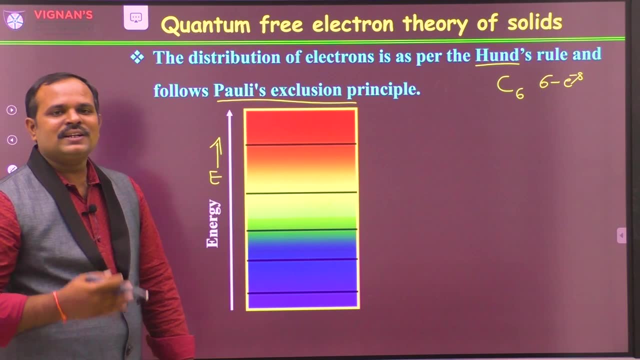 energy level. You can see this color changing means there is a continuous energy levels. However, for simplicity, just to understanding purpose, I am considering these are the sum of the energy levels. out of all these continuous energy levels, Now I have a system of carbon. 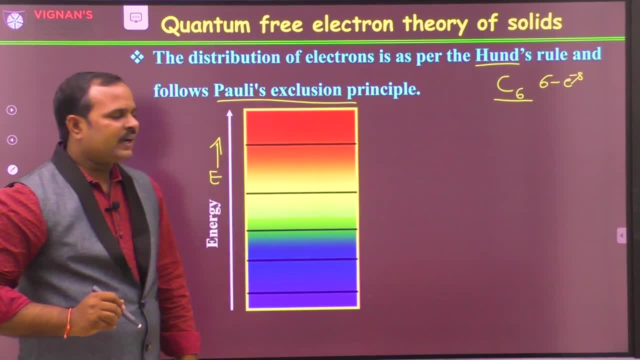 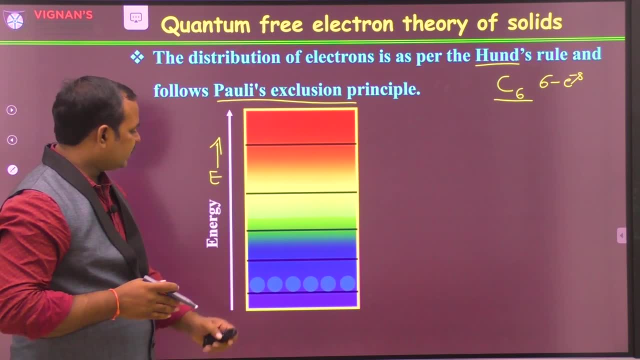 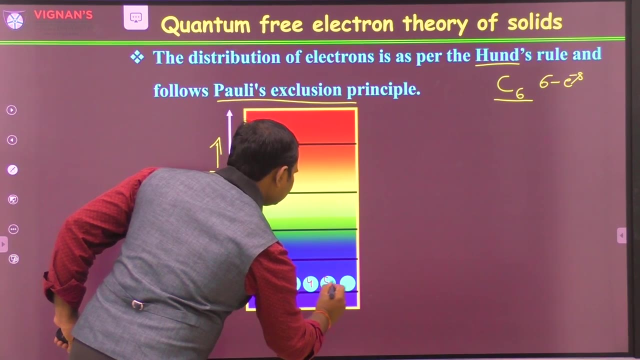 atom, where six electrons are there. According to classical mechanics, how these six electrons are going to be distributed among all these energy levels? It is like this way: There are six electrons. are there One, two, three, four, five, six? All these six electrons can be in one particular state. 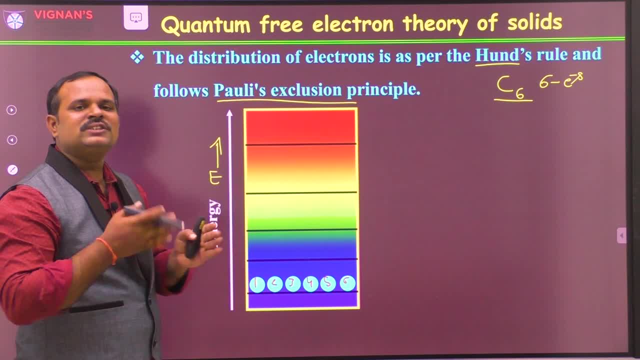 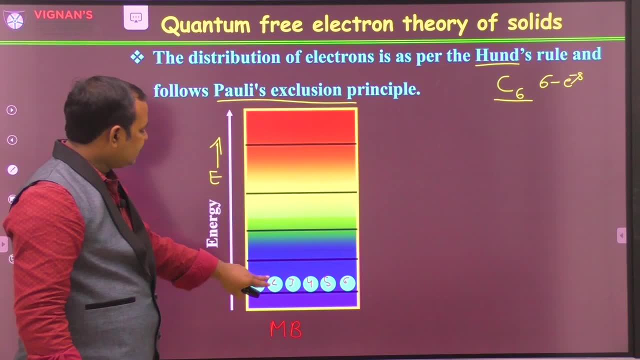 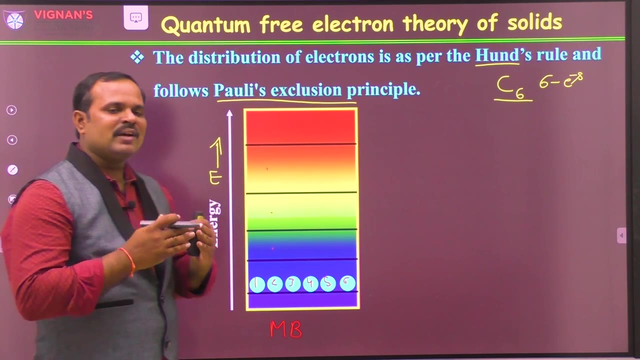 There is no restriction on the distribution of electrons. according to Maxwell-Boltzmann statistics, It can be even here, here, here, anywhere. There is no restriction on where the number of electrons should be there and how many number of electrons should be there in a particular. 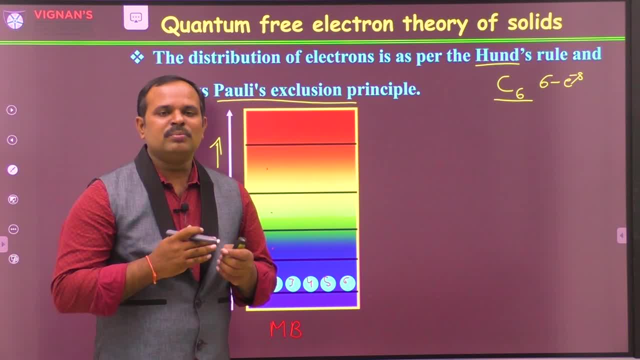 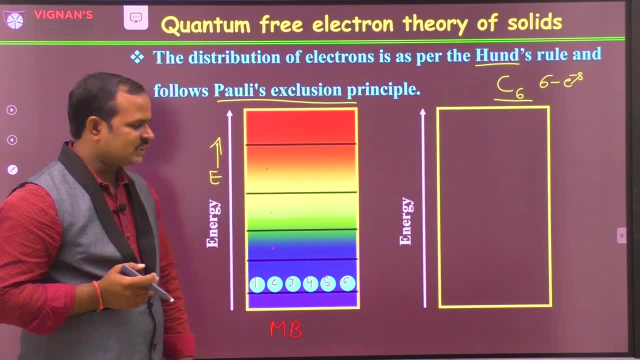 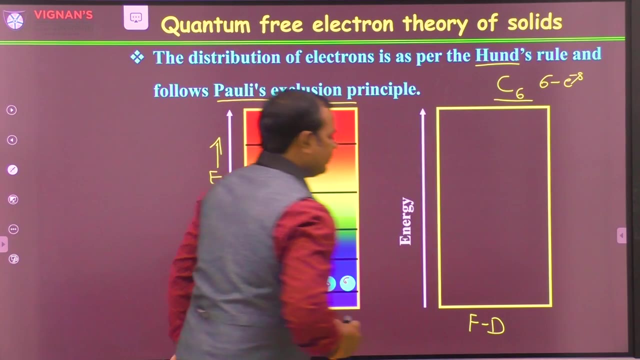 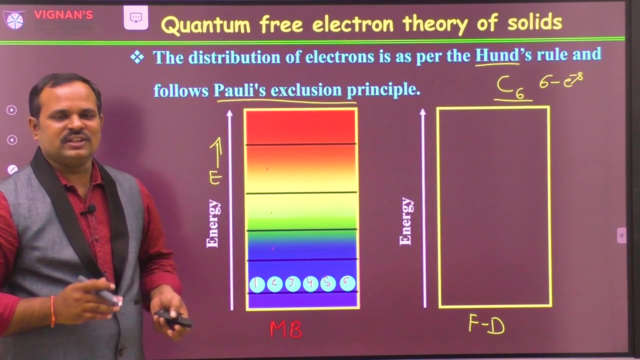 energy level because of the classical Boltzmann statistics. However, when it comes to the quantum mechanics, there is a Fermi-Dirac distribution function, Fermi-Dirac statistics. We know that, according to quantum mechanics, the energy is not continuous, it is discrete. 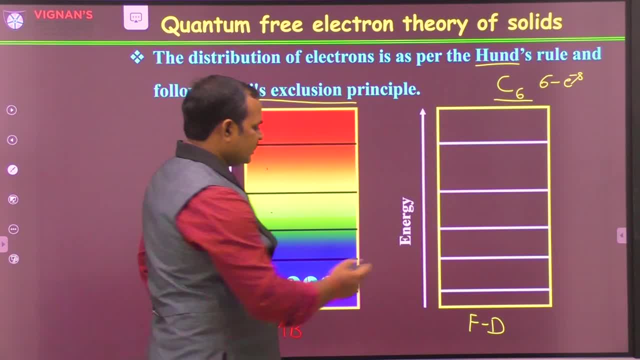 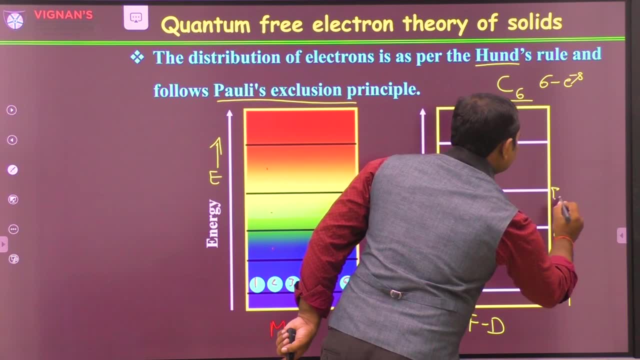 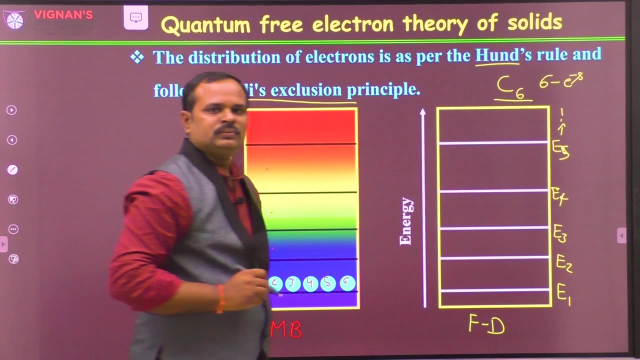 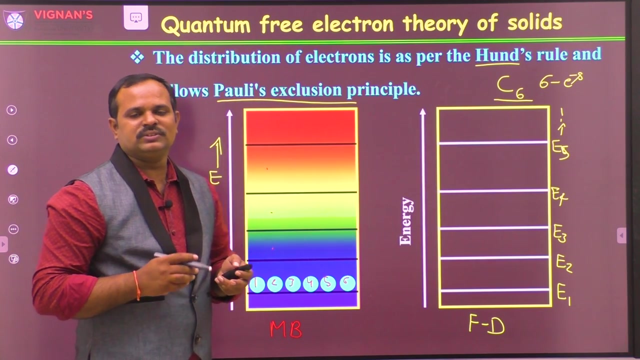 So we have discrete energy levels. All these are discrete energy levels with different energy: E1, E2, E3, E4, E5 and so on. Now how these six electrons in the same carbon atom, according to Fermi-Dirac statistics, can be distributed. 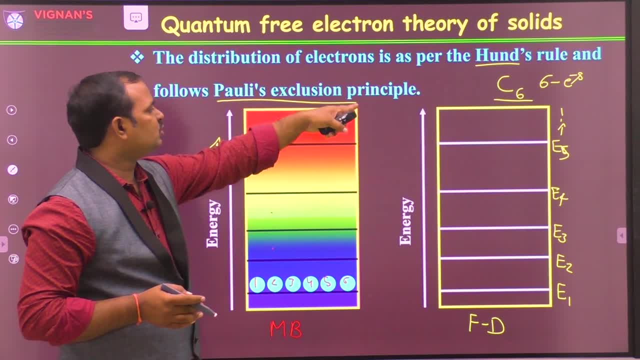 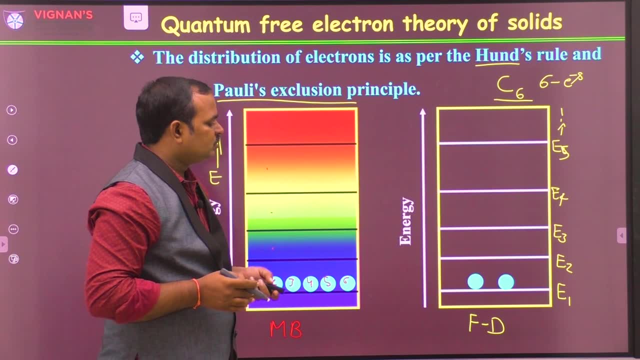 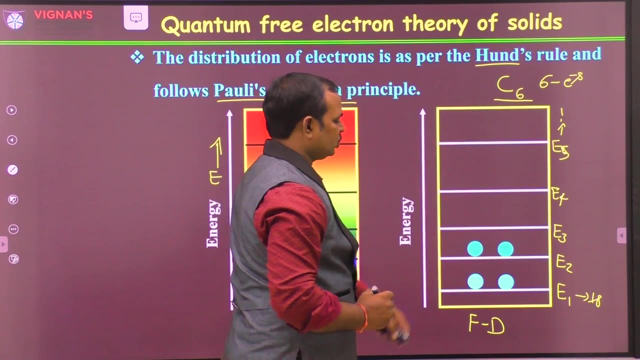 Certainly this has to be follows a Hund's rule as well as follows exclusion principle. Now, according to Hund's rule, the electrons will go into the first energy level. This is maybe we can consider 1s, and the next two electrons will go to 2s, because two next 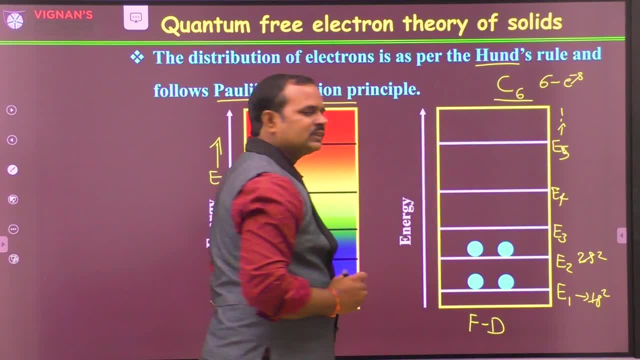 to sub level. This is 1s2, 2s2.. And then next two electrons will go to 2s. And then next two electrons will go to 2s. And then next two electrons will go to 2s. 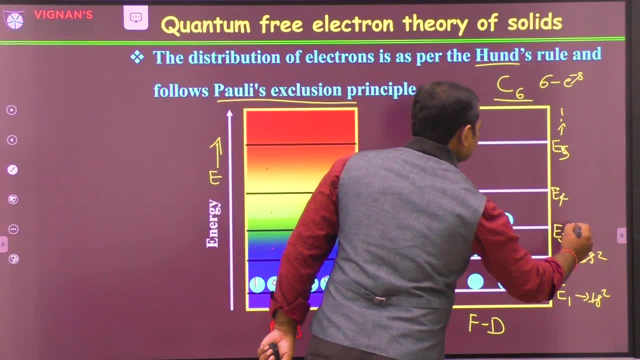 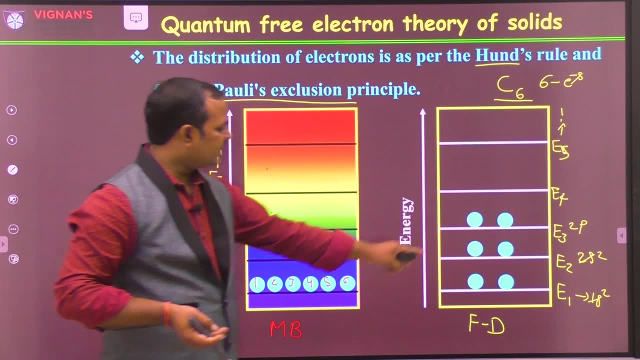 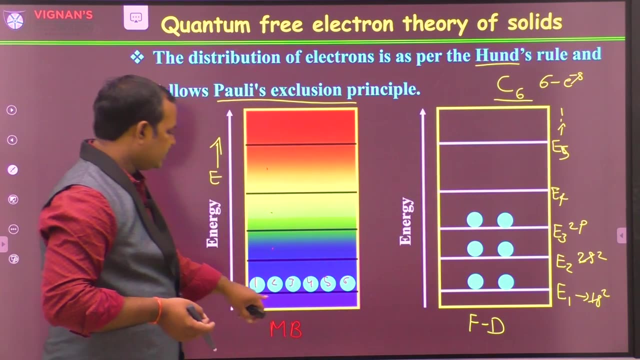 And then we will go to next energy level, that is, 2p sub level. This is how the electrons will be distributed. Now you can see all these six electrons. no two electrons will have the same four quantum numbers. But here you can see, all of them can be in one single state or they can be distributed. 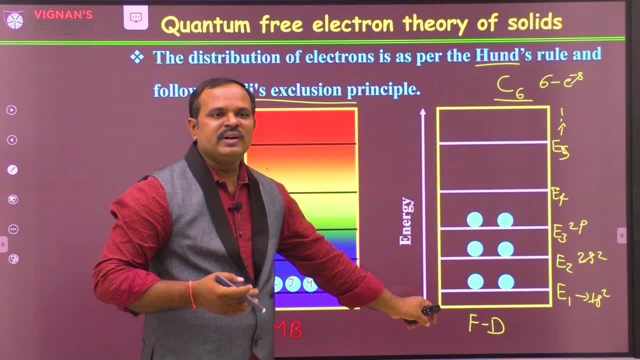 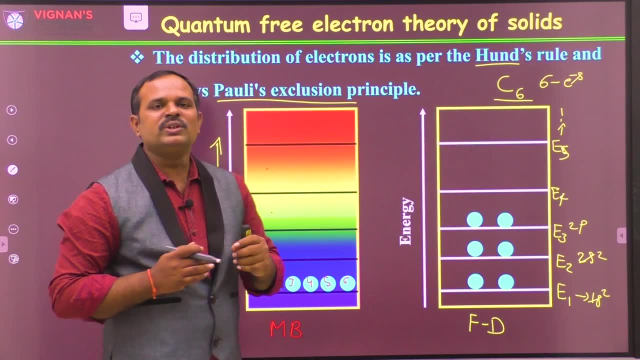 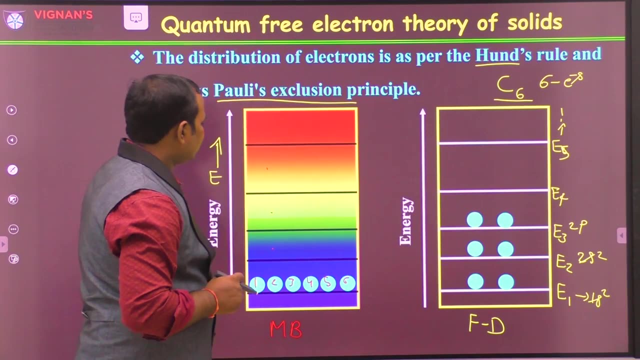 any number of electrons in any state, But according to Fermi-Dirac statistics, the electrons are fermions and then they have to follow Hund's rule and also Pauli's exclusion principle. Now, in this way the electrons are distributed. What is the use? There is a use here, If you remember our specific heat and many other. 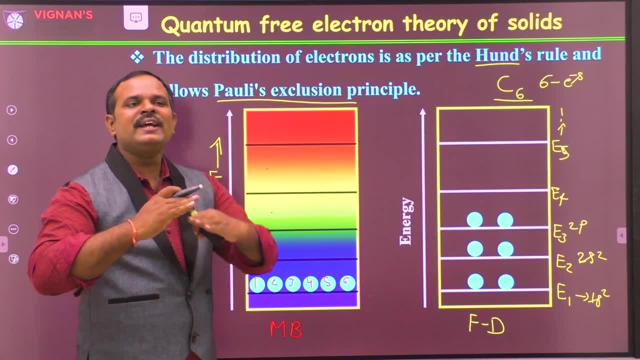 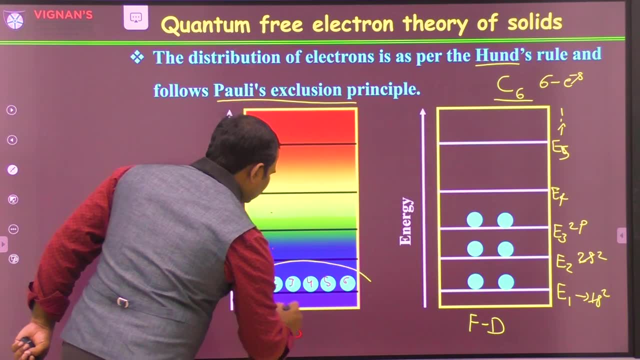 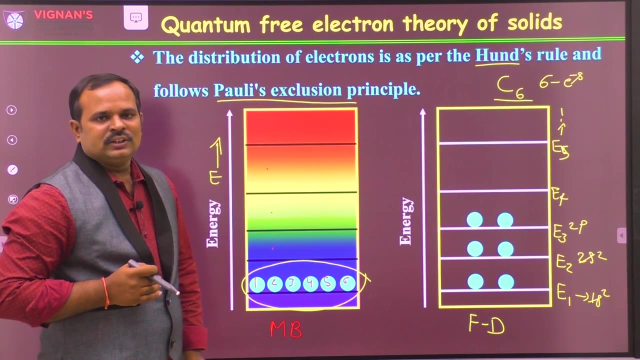 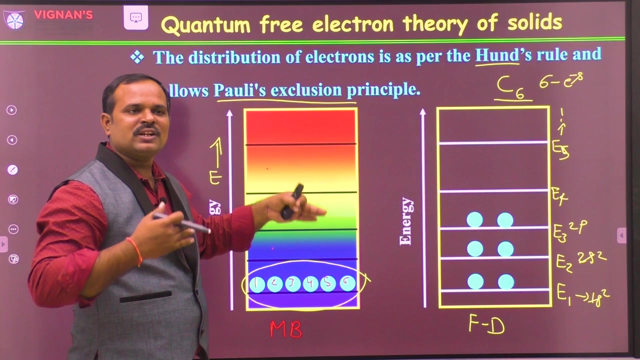 experiments where the classical mechanics got higher number of values. That is because in the classical mechanics they consider all these electrons. all of them are participating in the conduction process or the respective process. That is reason why the specific heat got more number and many other properties also got higher numbers and also wrong values. However, electrons 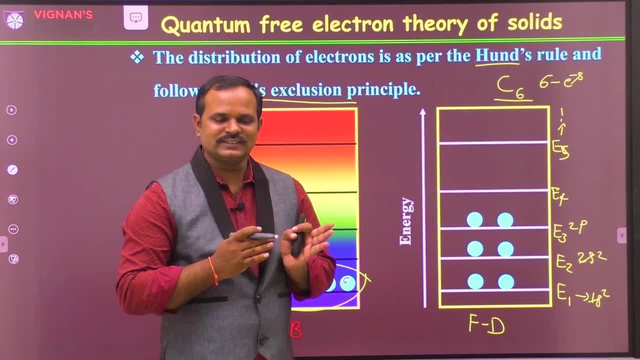 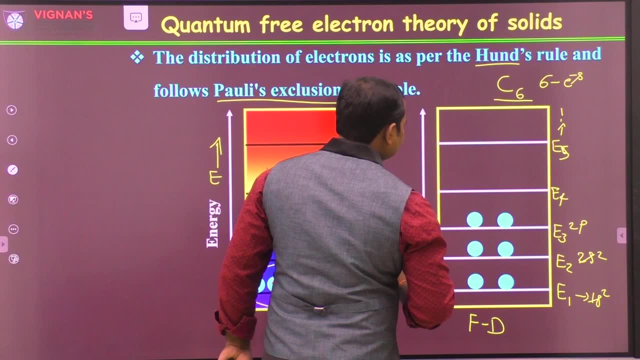 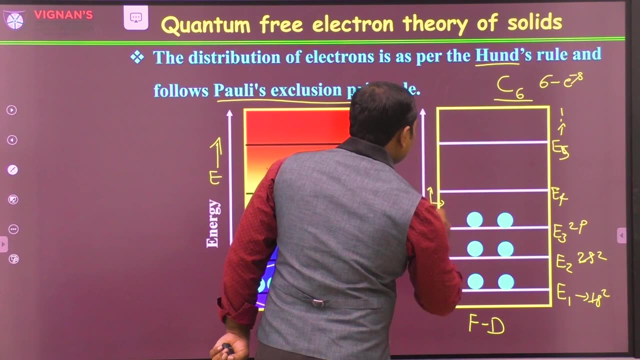 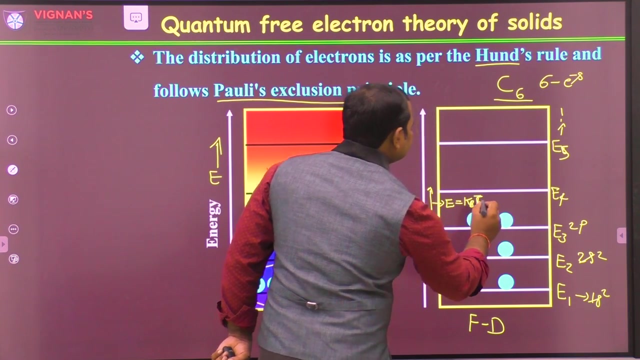 are fermions and then they follow Fermi Dirac statistics. So now, according to this one, this is the distribution. Now, what is the use of this one is, In the quantum free electron theory, what they consider Only those electrons which are in the range of E is equal to KBT, where T is temperature. Only those. 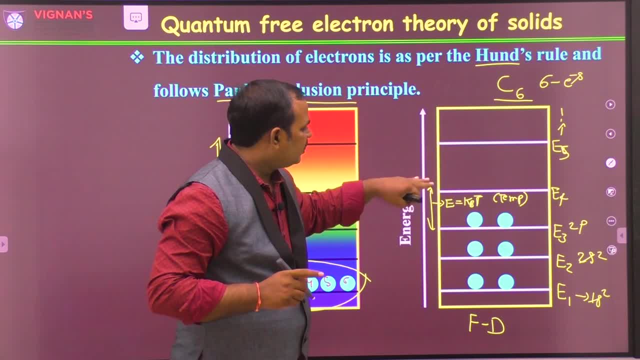 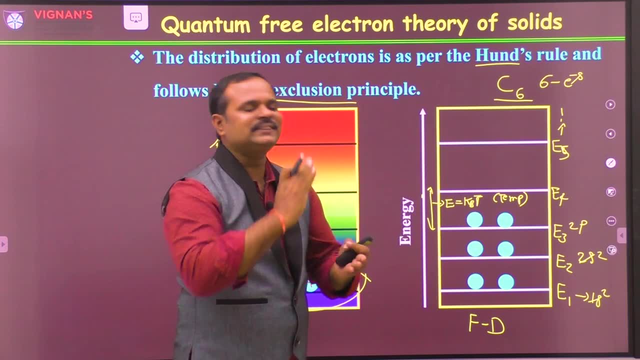 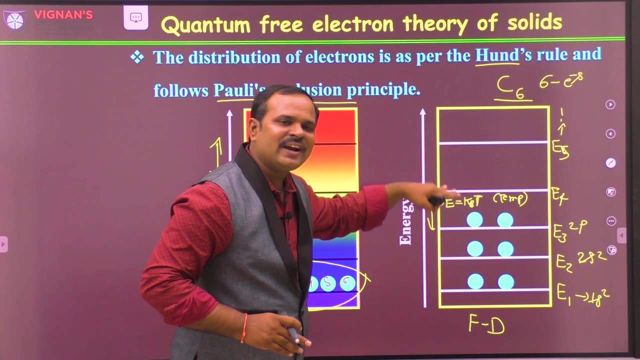 electrons which are participating into the process are from the top most free energy level to the KBT range. That means the thermal energy which can excite the electrons are in the KBT range Only, not the other electrons, So that only a fraction of electrons can be participated in the 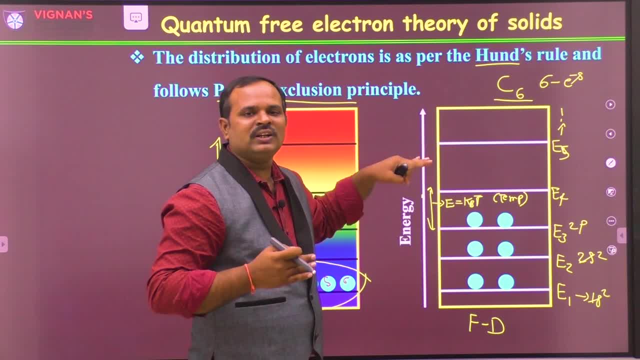 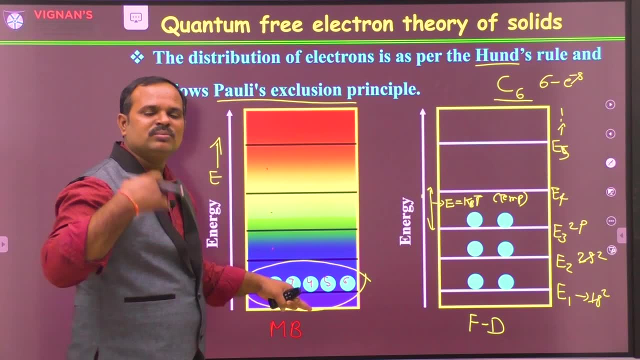 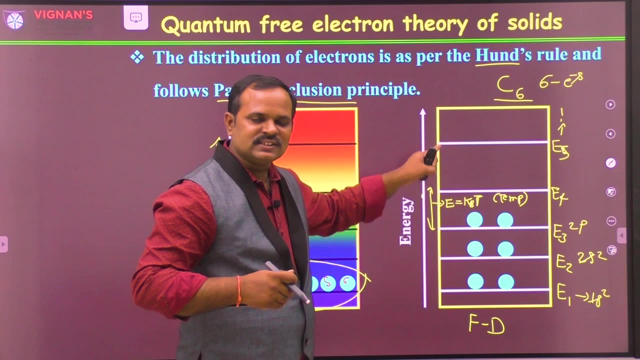 conduction process or any the respective process, So that they can give exact amount of information. But here, in this case, all the six electrons are participated, So you get more number of more, more in a number in every physical property. But here they consider like: this way You will see all these. 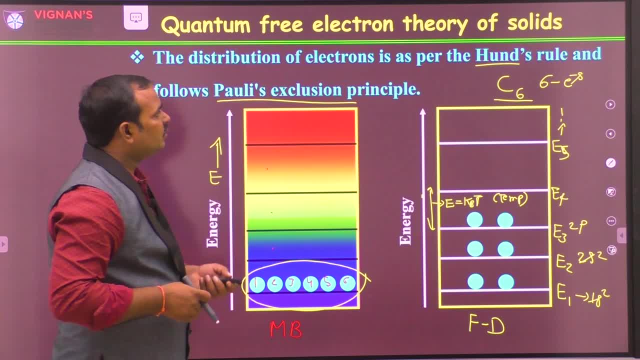 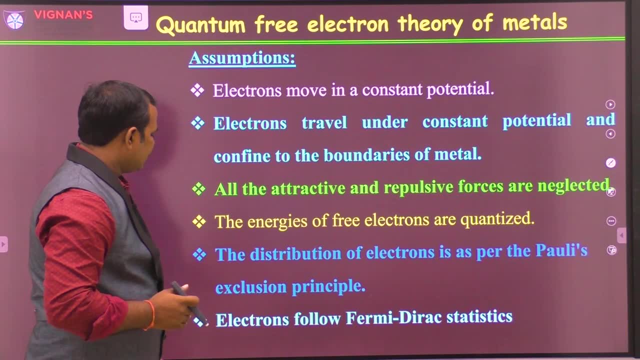 things in a subsequent classes. This is about the distribution of electrons. One thing is that the distribution of electrons is not the same as the distribution of electrons. So the distribution of electrons- electrons according to Pauli's exclusion principle and Hund's rule. Next Electrons follows Fermi-Dirac. 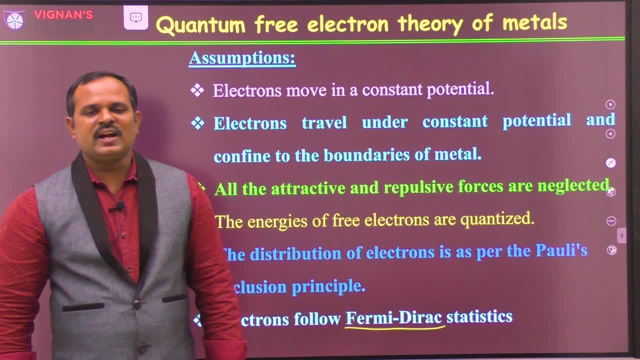 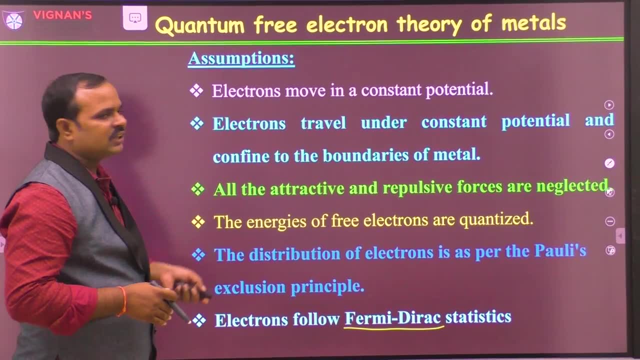 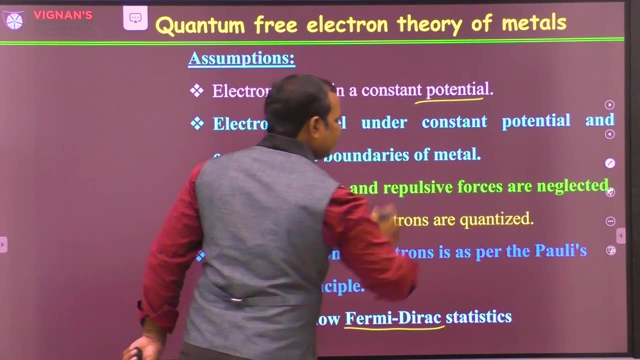 statistics. Electrons also follows Fermi-Dirac statistics. This you will see more clearly in the next class. So these are the assumptions of the quantum free electron theory. The first one is: electrons moves in a constant potential. This is the same as a classical free electron theory. 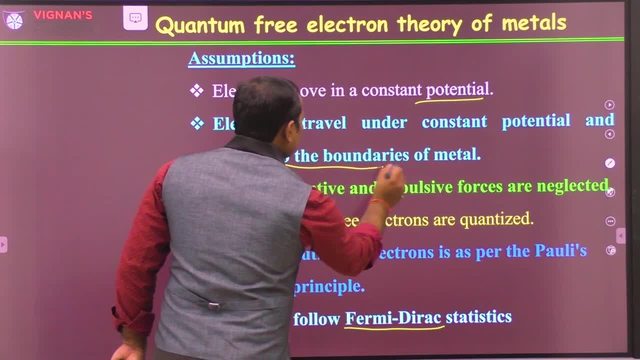 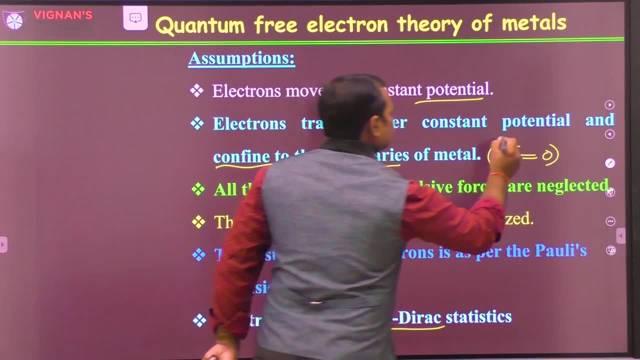 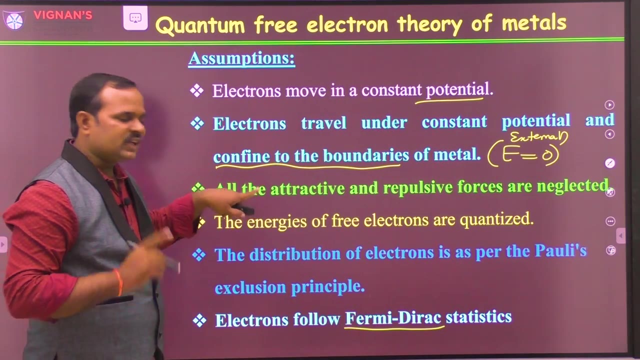 and then they, all these electrons, are confined to the boundaries of the metal. under electric field is zero. Applied electric field is zero. External electric field. All these, all the attractor and refulsive forces are neglected. and the next one is the energies. 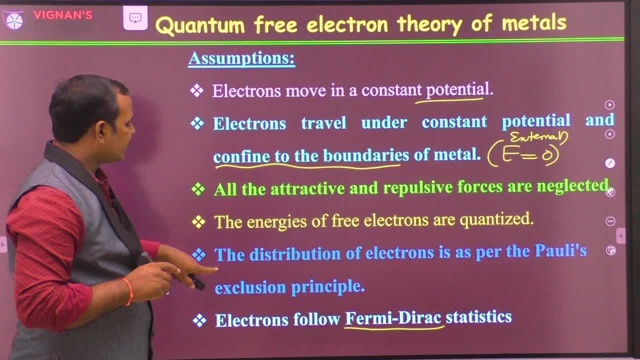 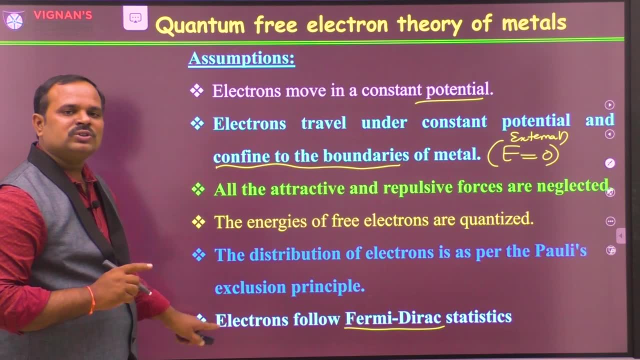 of the free electrons are quantized And the next one is the distribution of electrons are as per the Pauli's exclusion principle and Hund's rule, And electrons follows Fermi-Dirac statistics. Thank you so much.